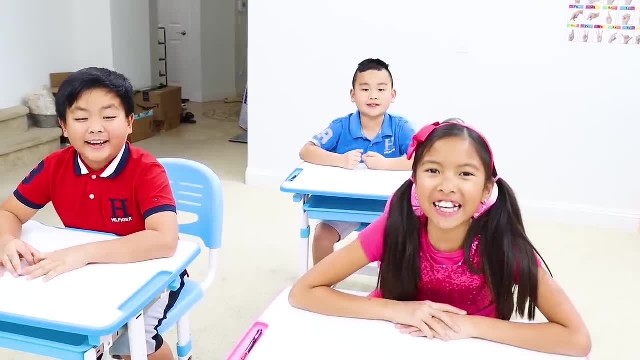 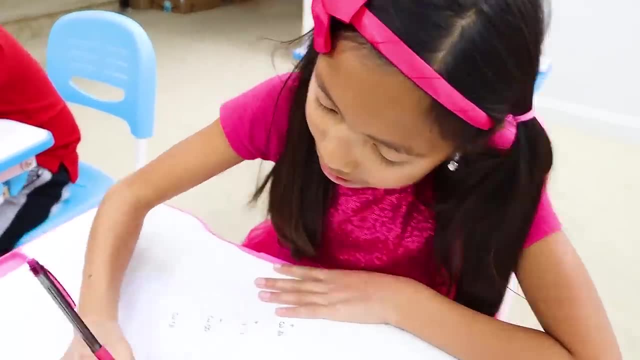 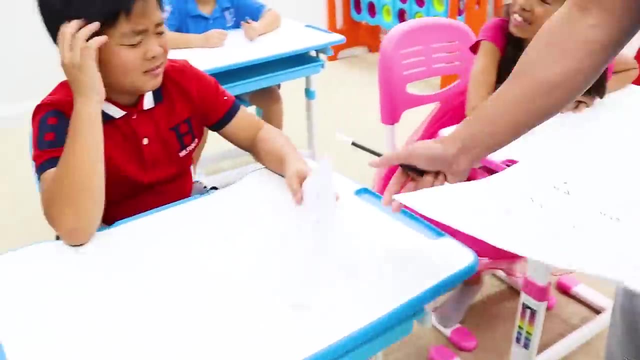 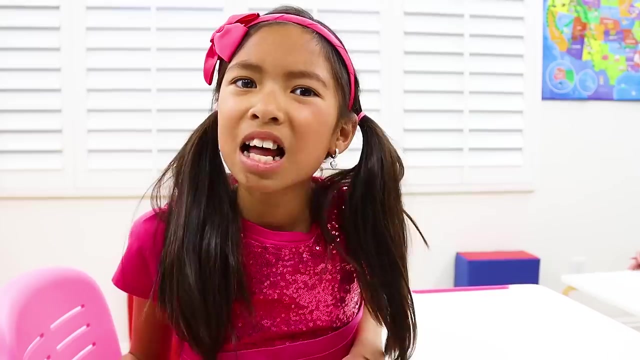 Are you ready for the test? Yes, we're ready. Okay, good, Let's start. Thank you. Thank you, Uncle Jay. Time's up guys. Okay, let me go check. Let's see. Alex, I think you won't pass. 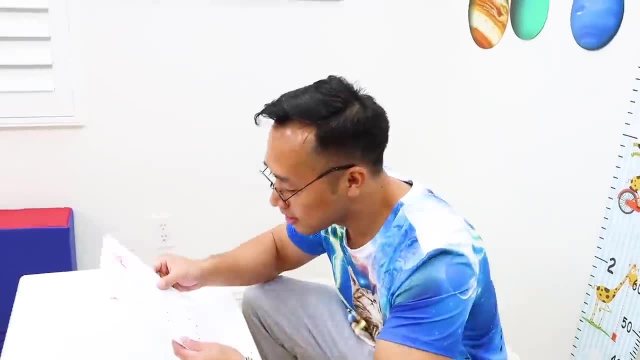 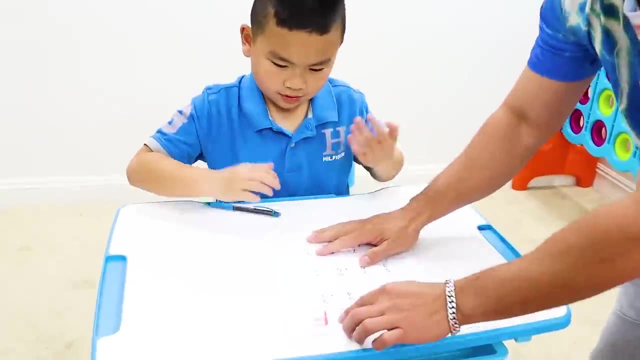 I don't think so, Wendy. I think I want to get an A. Okay, I'm all done. Here's your test, Wendy, Thank you. Here's your Alex And here's your Lyndon. Oh no, I got an F. 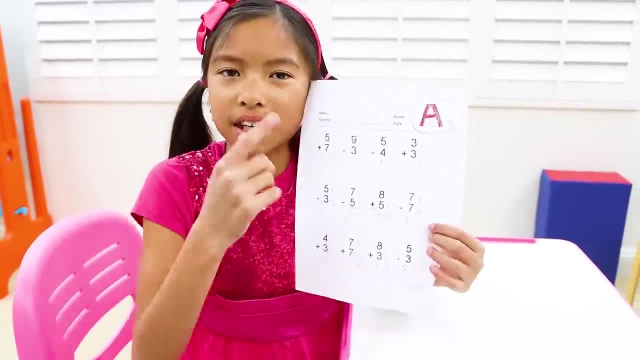 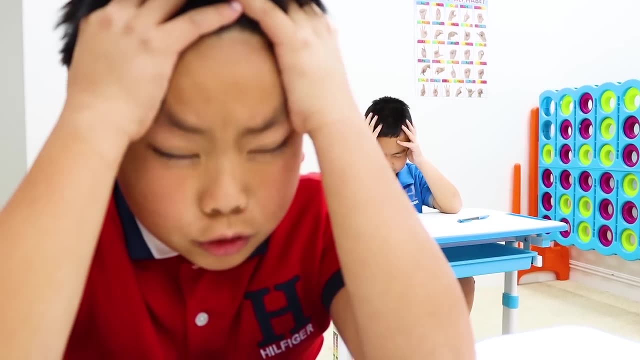 Me too. I told you, Alex, I'll get an A Na na na, boo, boo. Bye, What am I going to do? Hey, Alex, Uncle Kay can teach us math. Do you want to go? 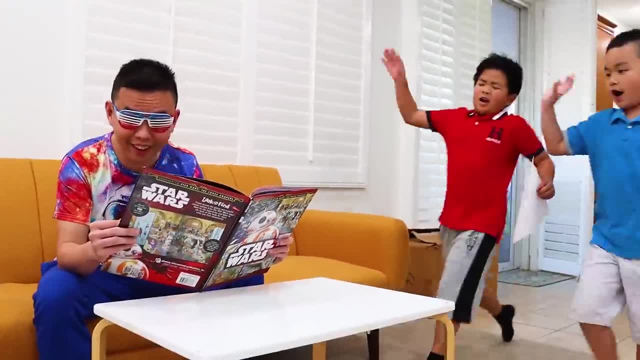 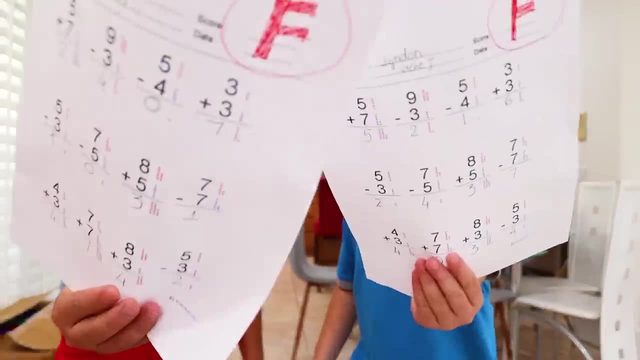 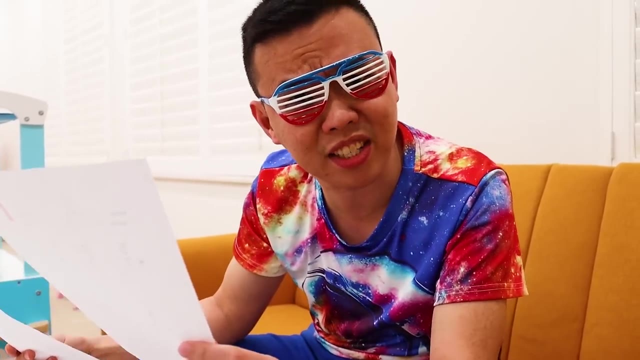 Sure, let's go. Okay, Uncle Kay, Uncle Kay, What happened? guys? Can you teach us how to do math? No problem, but let me see your test first. Here you go, Hmm, let me see. Hmm. now I can see you guys have the same problem about the minus and plus sign. 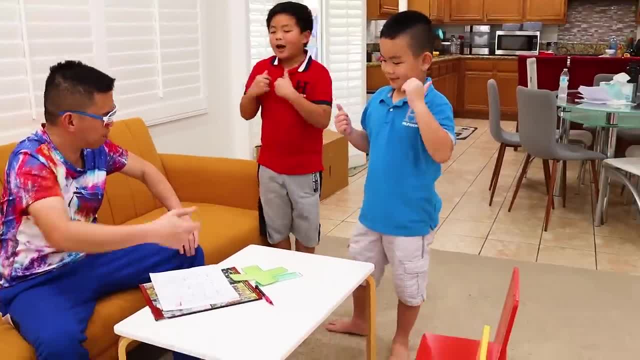 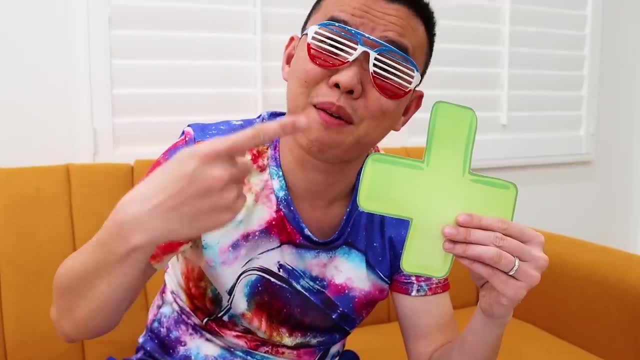 Uh-oh, Don't worry, Just sit down here. Okay, Look guys, This is the plus sign. What does it mean? Plus sign means addition. Still not get it? Ah, just wait here, Hey guys Look. 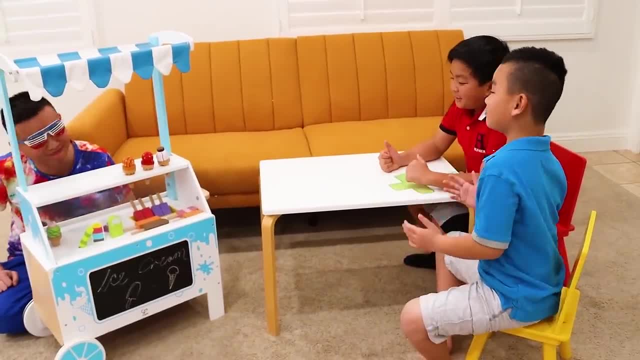 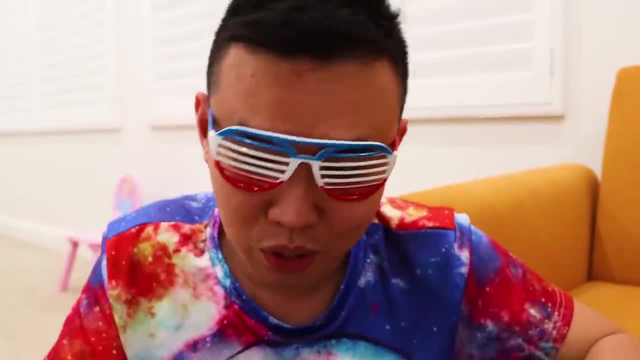 Wow, ice cream. Now I'm going to give two ice cream for Lyndon. Thank you, Uncle Kay. Ooh, And now two popsicles for Alex. Thank you, Uncle Kay. Wait, wait, wait, wait, Don't eat yet. 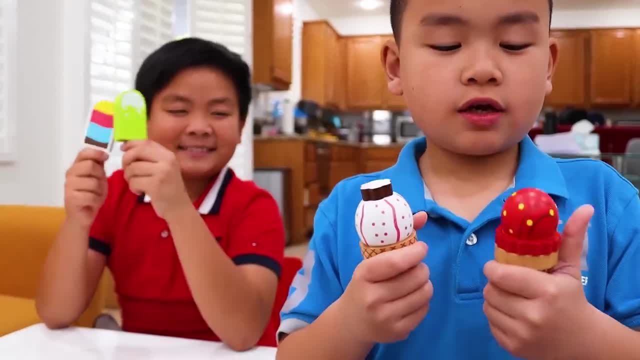 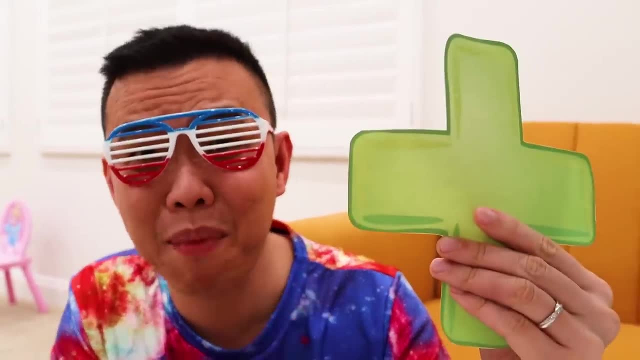 Let's count the ice cream both of you have, Okay, Uncle Kay, One, two, three, four, Four. Uncle Kay, That's correct. That's what plus sign means. Yeah, I got it now. It's so easy. 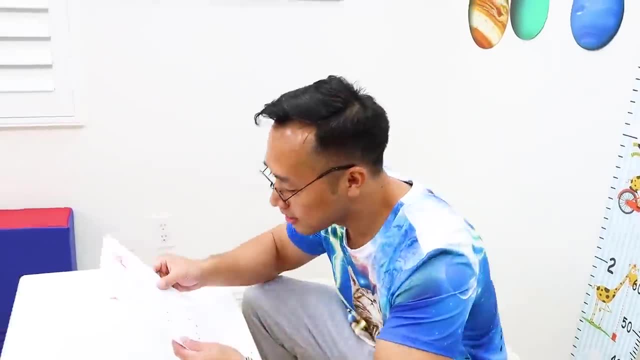 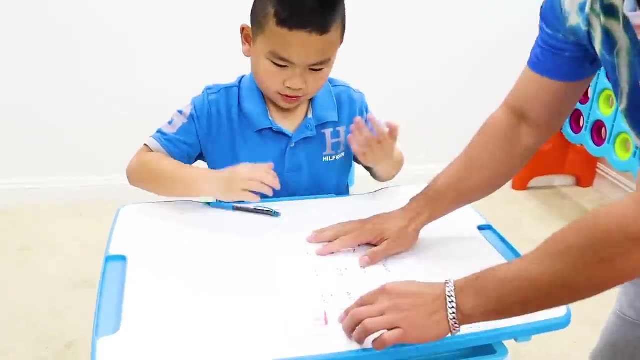 I don't think so, Wendy. I think I want to get an A. Okay, I'm all done. Here's your test, Wendy, Thank you. Here's your Alex And here's your Lyndon. Oh no, I got an F. 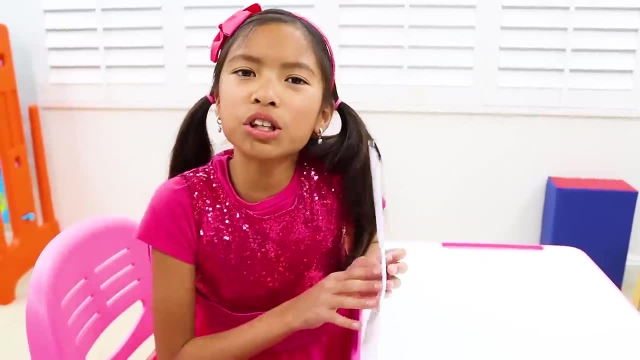 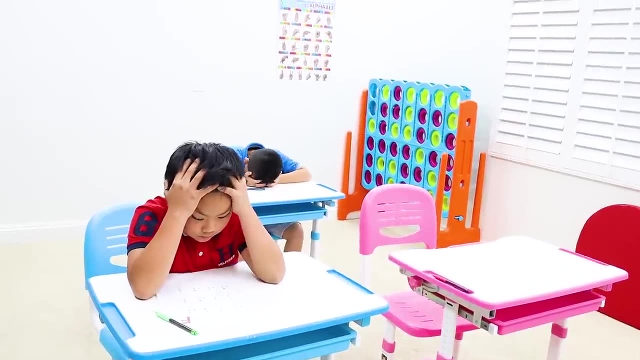 Me too. I told you, Alex, I'll get an A Na na, na na, boo, boo. Bye. What am I going to do? Hey, Alex, Uncle Kay can teach us math. Do you want to go? Sure, let's go. 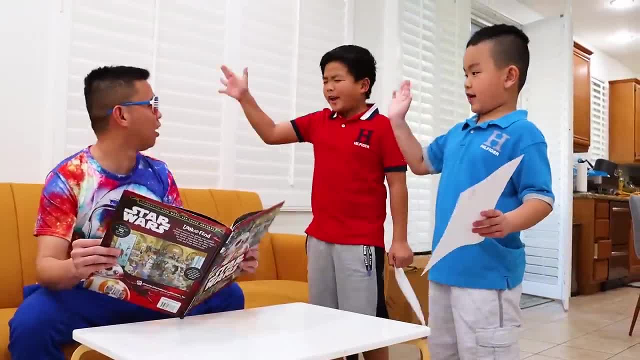 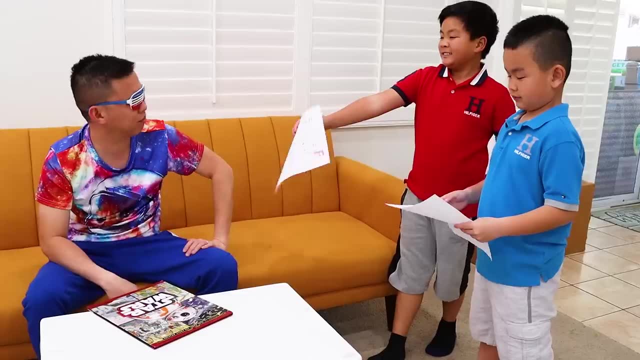 Okay, Uncle Kay. Uncle Kay, What happened? guys, Can you teach us how to do math? No problem, But let me see your test first. Here you go, Hmm, let me see, Hmm. now I can see you guys have the same problem about the minus and plus sign. 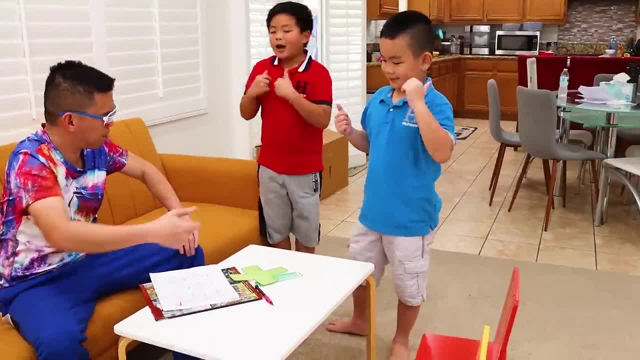 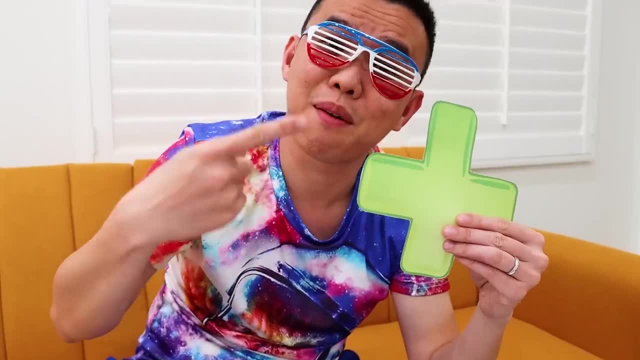 Uh, oh, Don't worry, Just sit down here. Okay, Look guys. This is the plus sign. What does that mean? Plus sign mean addition. Still not get it. Ah, just wait here, Hey guys Look. 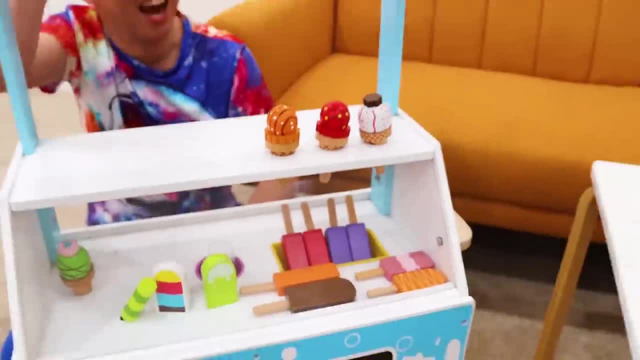 Wow, ice cream. Now I'm going to give two ice cream for Lyndon. Thank you, Uncle Kay Woo. And now two popsicle for Alex. Thank you, Uncle Kay. Wait, wait, wait, wait, Don't eat yet. 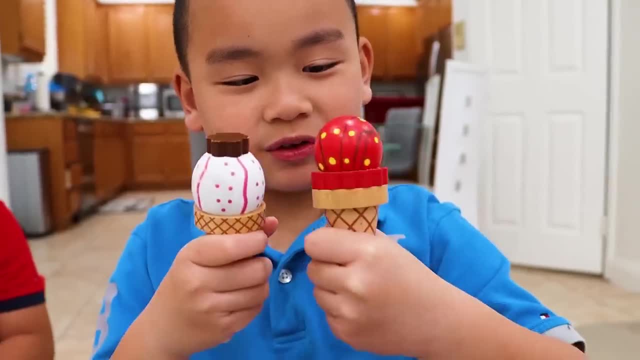 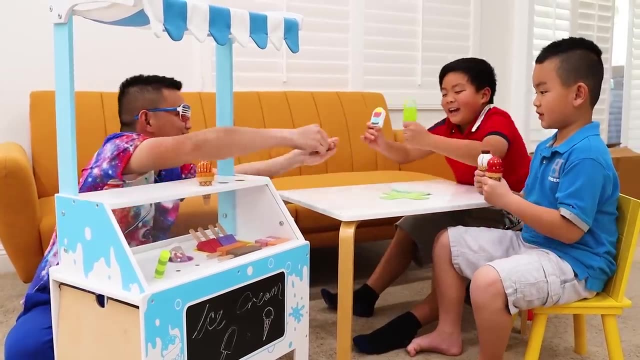 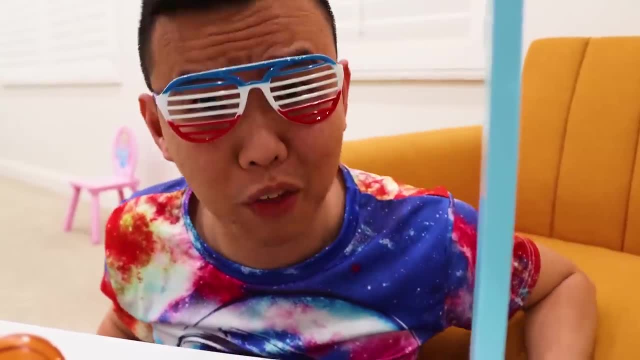 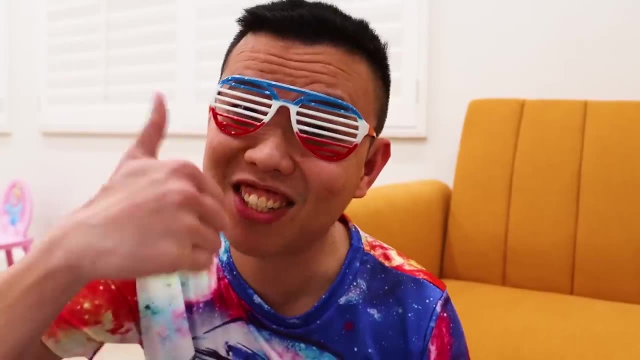 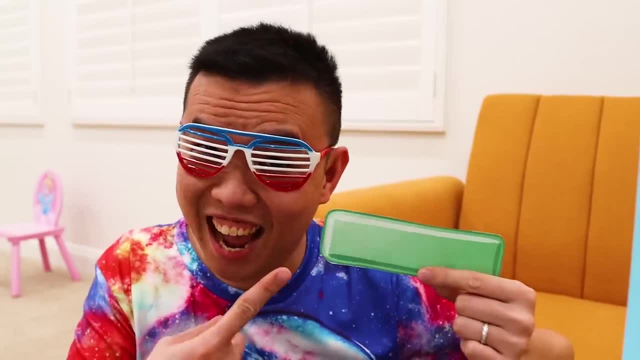 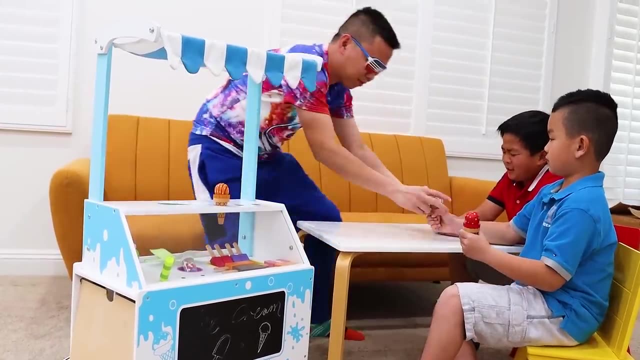 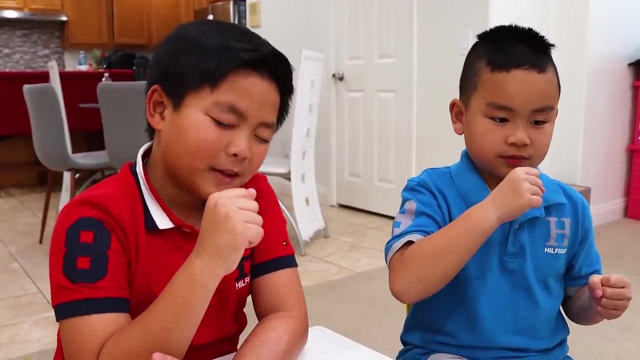 Yeah, I got it now, It's so easy. And now this is the minus sign. What does it mean? Let me show you. Huh, Now eat your ice cream. Okay, Uncle Kay, We're done, Uncle Kay. 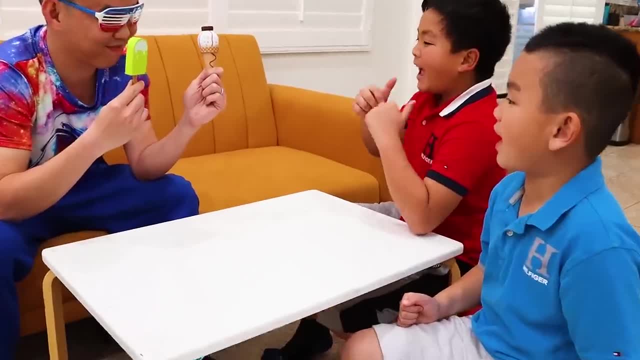 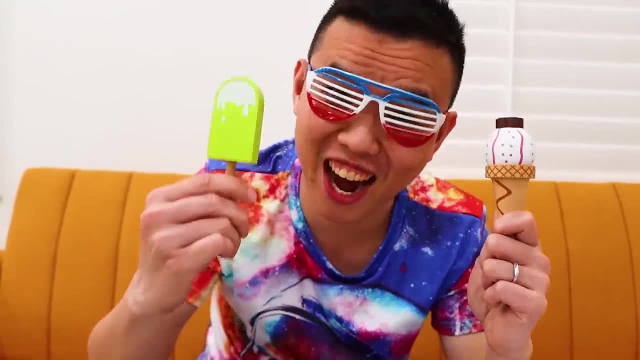 Now count how many ice cream I have left. Okay, One, two. It's two ice cream, Uncle K. Good job, You guys got it now. Thank you, Uncle K, You're welcome. We have to go now. 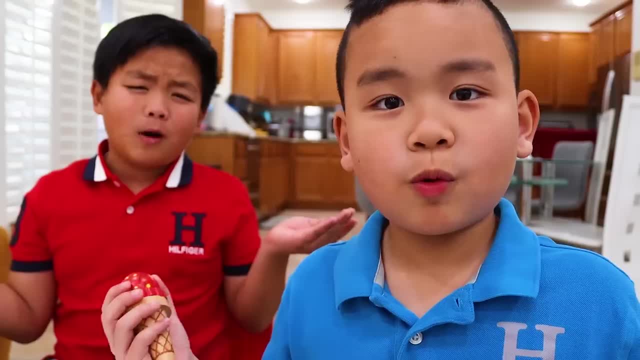 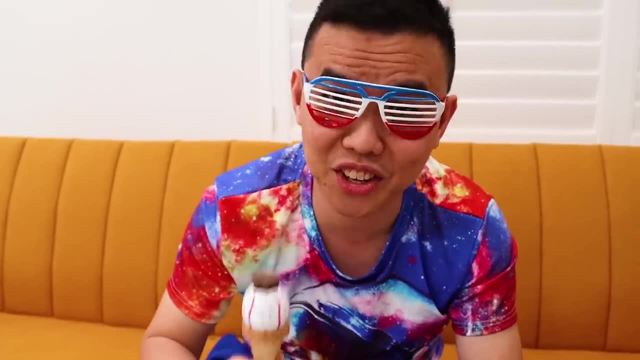 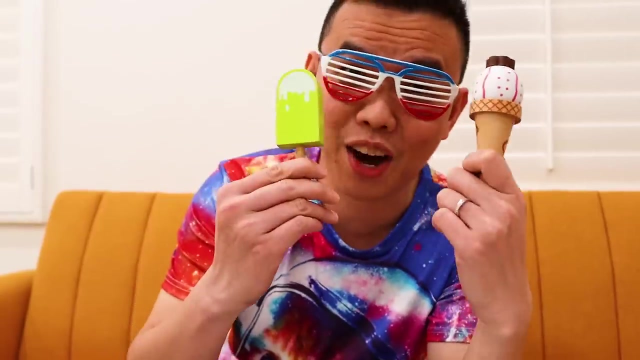 And now this is the minus sign. What does it mean? Hmm, let me show you. Huh, Now eat your ice cream. Okay, Uncle Kay, We're done. Uncle Kay, Now count how many ice cream I have left. 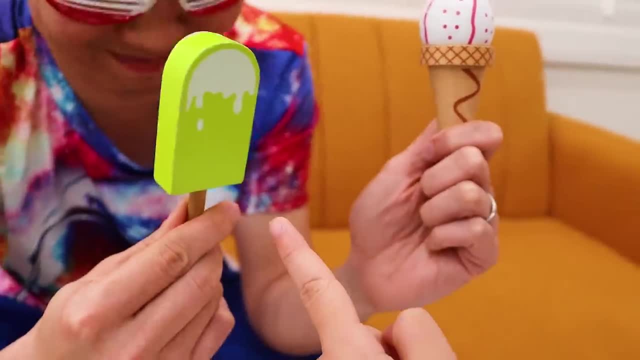 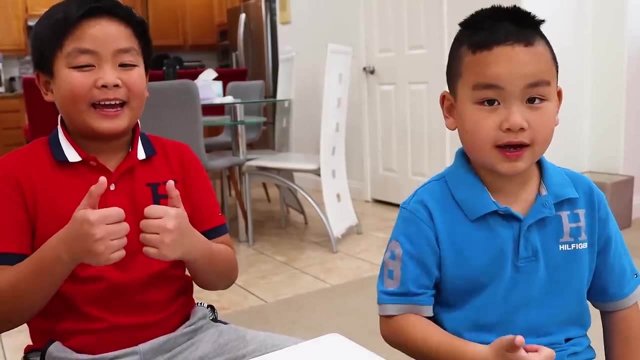 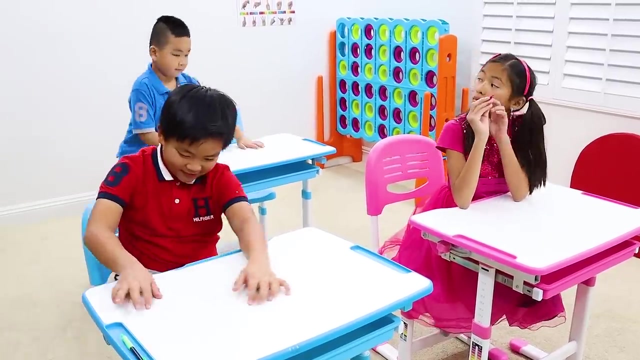 Okay, One, two, It's two ice cream, Uncle Kay. Good job, You guys got it now. Thank you, Uncle Kay. You're welcome. We have to go now, Bye, Bye. Hey, Alex, Are you ready to get an F? 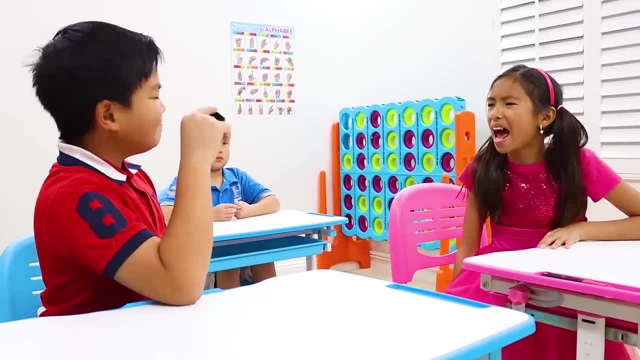 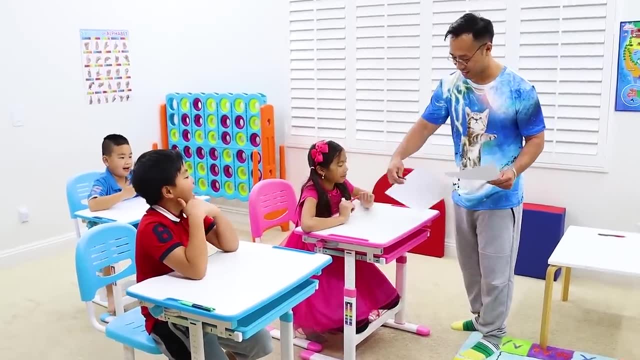 I don't think so, Wendy. Hmm, I think you'll get an F. That's not nice, Alex. do your best, Let's see. Alex, Are you guys ready for the test? Yeah, Here you go, Wendy. 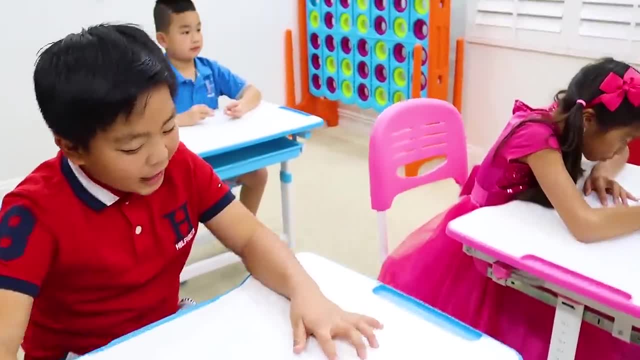 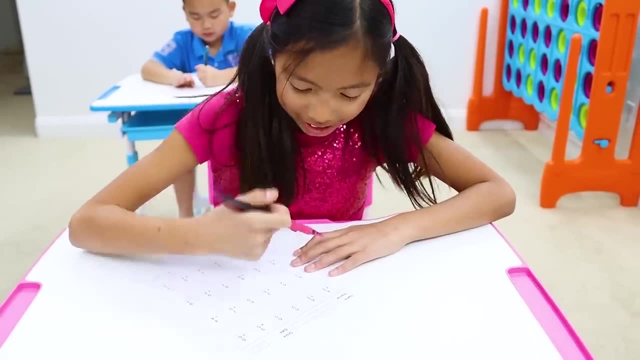 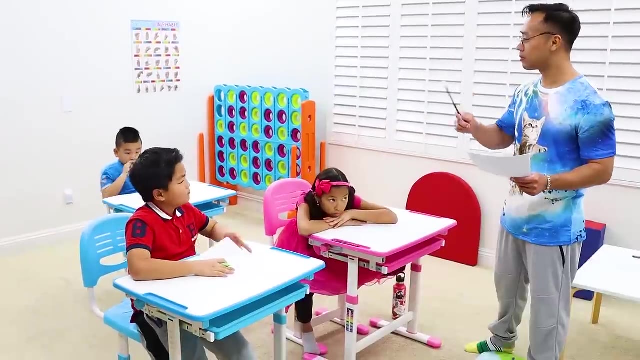 Thank you. Here you go Alex. Thank you, Uncle Jay, And here you go Lyndon. Thank you, Okay, you have 30 minutes starting now. Okay, I'm done, Uncle Jay. Good job, Wendy. Okay, guys, thumbs up. 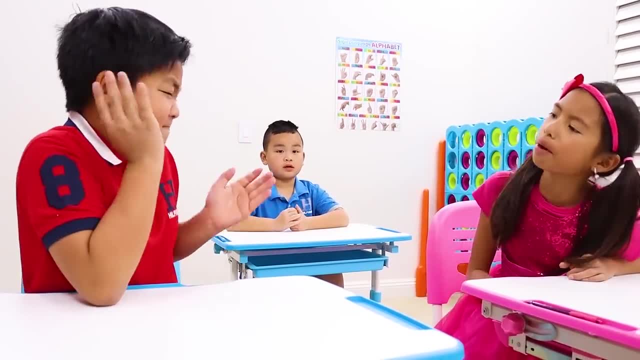 Alex. I finished before you guys. I'm going to still have an A, Alex, it will be fine. Okay, I'm all done checking. Here's your test, Wendy, You're going to get an F again. Here's yours, Alex. 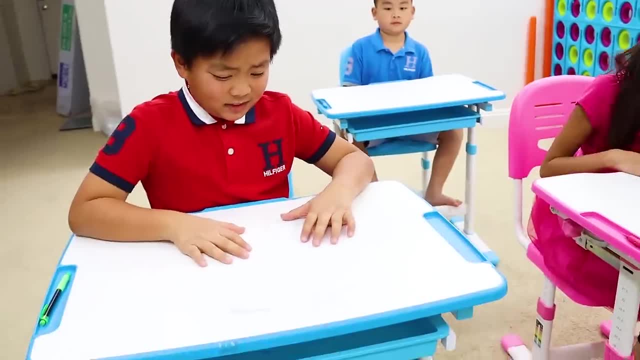 Whoa F again. right, I told you, No, I got an A. Look Me too, I got an A, Huh, Oh, no, I got a B, guys, Don't be sad, Wendy. 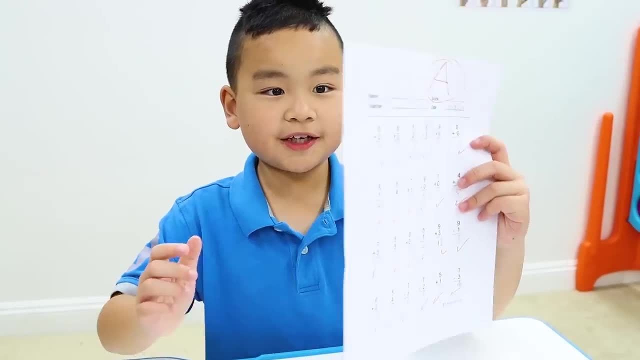 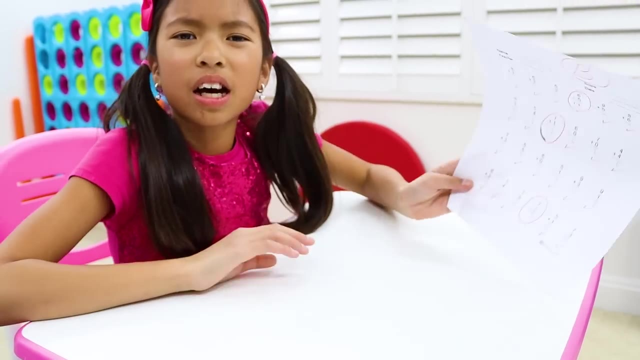 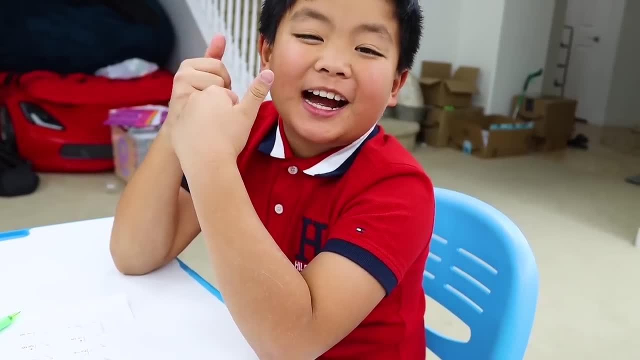 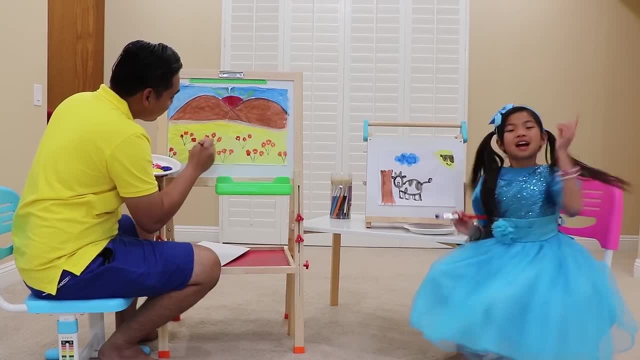 I don't mind. Thank you, Alex. Bye, Now let's use green to paint the tree guys. Oh no, What happened, Emma? I don't have any green for my painting. Uncle John, Don't worry, You can make it. Emma. 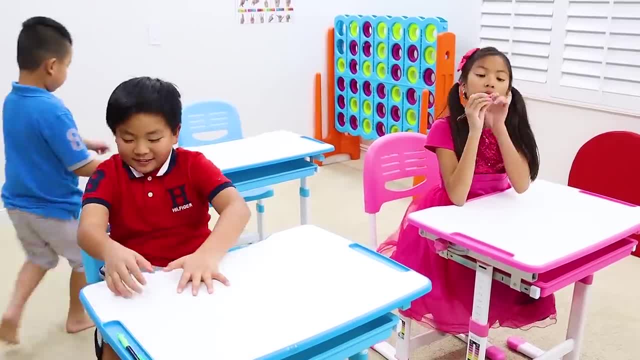 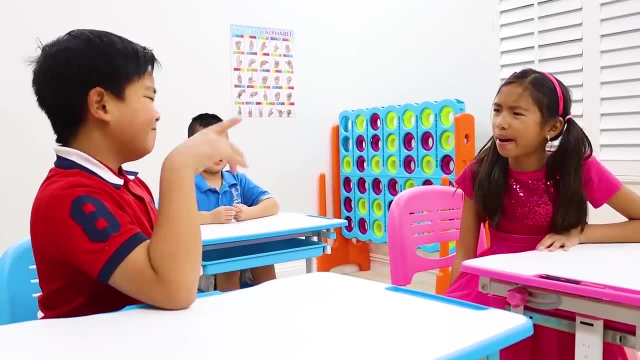 Bye. Hey, Alex, Are you ready to get an F? I don't think so, Wendy. Hmm, I think you'll get an F. That's not nice, Alex. do your best, Let's see. Alex, Are you guys ready for the test? 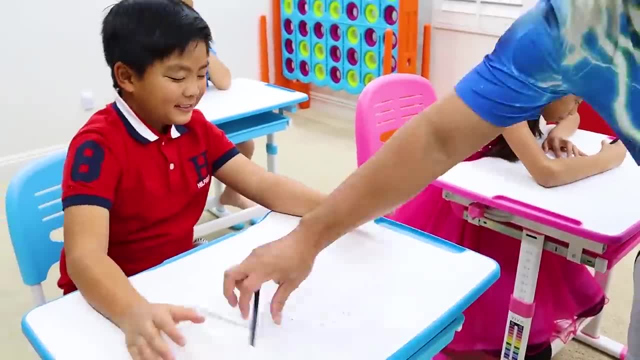 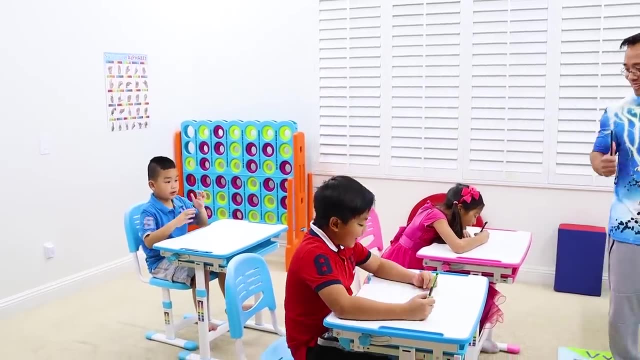 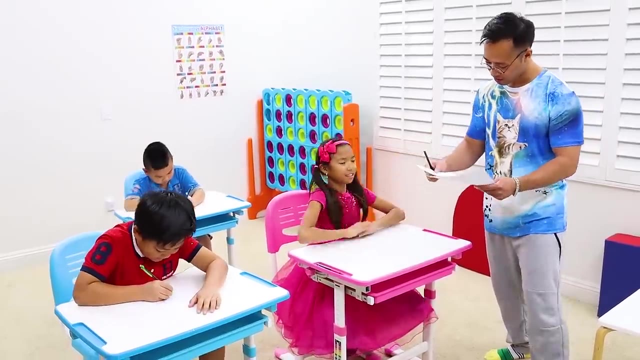 Yeah, Here you go, Wendy, Thank you. Here you go, Alex. Thank you, Uncle K, And here you go, Lyndon, Thank you. Okay, you have 30 minutes starting now. Okay, I'm done, Uncle K, Good job. 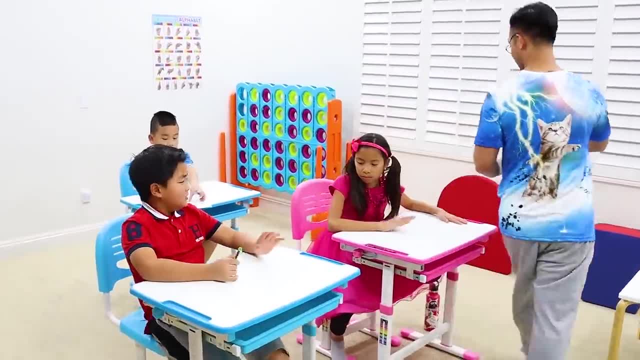 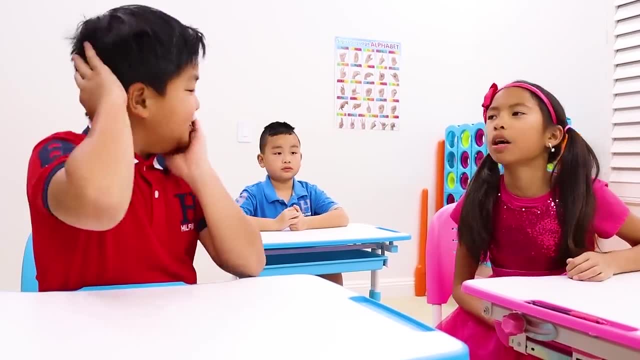 Wendy. Okay guys, thumbs up Alex. I finished before you, so I'm going to still have an A. Alex, it will be fine. Okay, I'm all done checking. Here's your test. Wendy, You're going to get an F again. 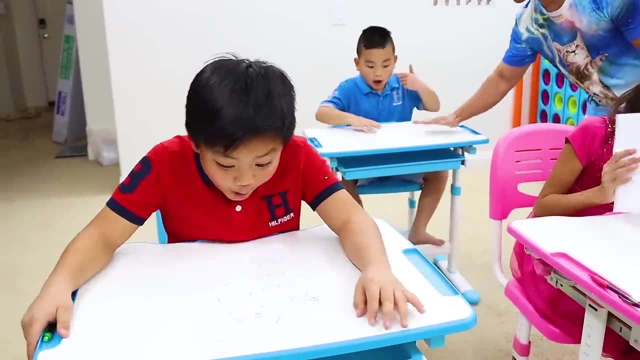 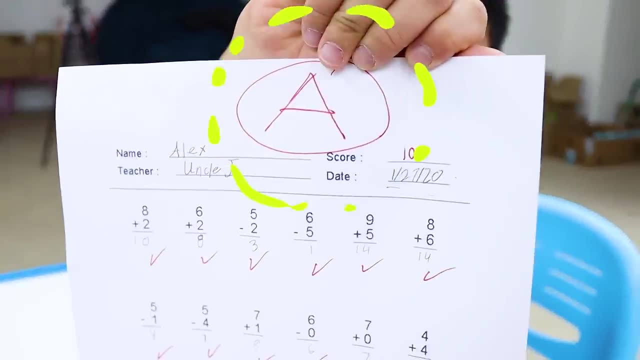 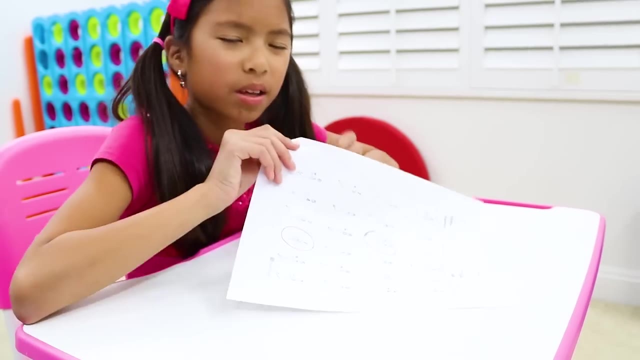 Here's your Alex Whoa F again. right, I told you, No, I got an A. Look Me too, I got an A. Huh, Oh, no, I got a B, guys. Don't be sad, Wendy, You can try again. 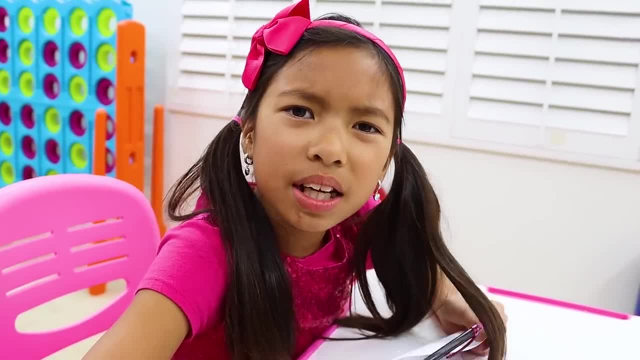 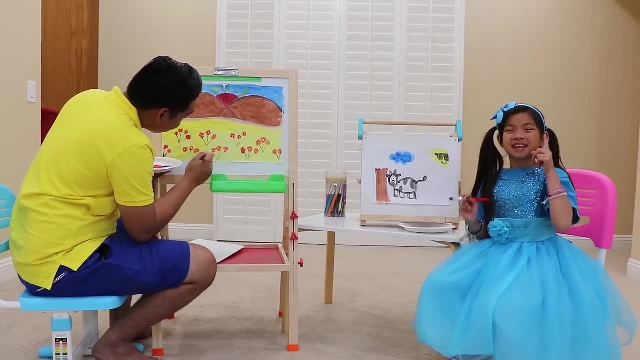 next time You're so nice. Sorry that I laughed at you earlier. It's okay, Wendy, I don't mind. Thank you, Alex. Bye, Now let's use green to paint the tree, guys. Oh no, Oh, What happened Emma? 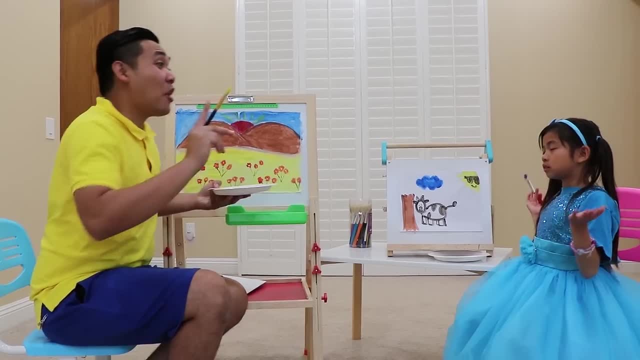 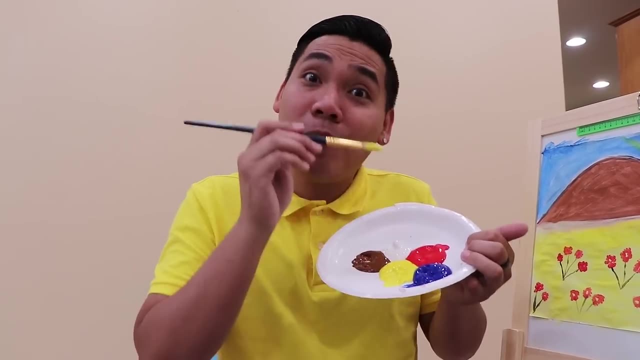 I don't have any green for my painting, Uncle John, Don't worry, You can make it. Emma, Really, Yeah, I'll show you. Thank you. You can make green from mixing yellow and blue. Let me show you. 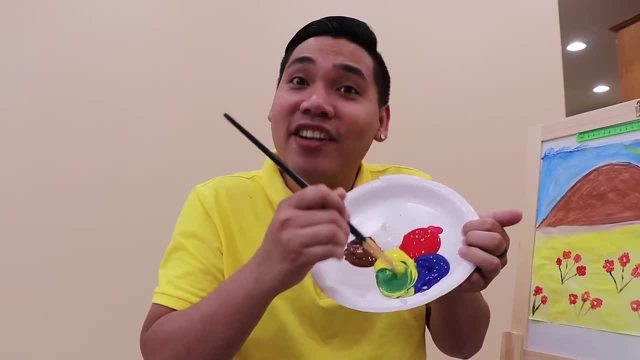 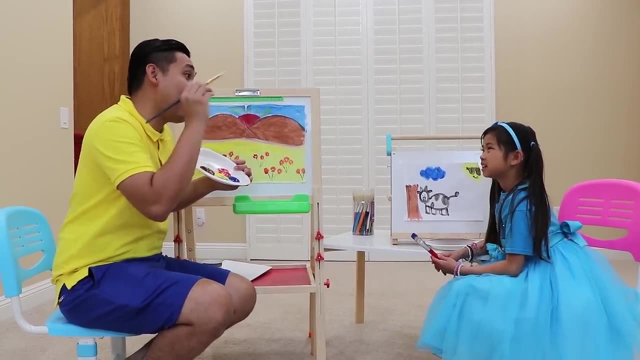 Look Awesome. See, It's turning green. Wow, Yeah, You can make more colors. If you mix yellow and red, you'll get orange, And if you want to make purple, you can mix red and blue. Let me show you. 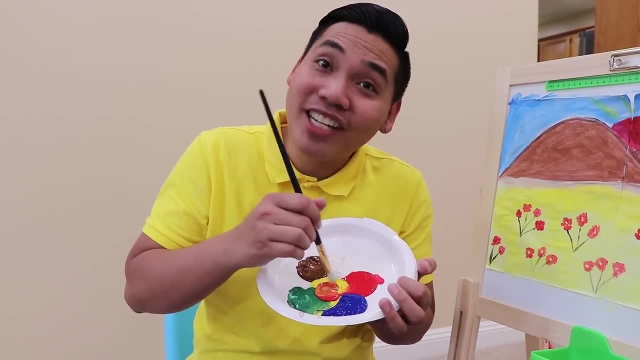 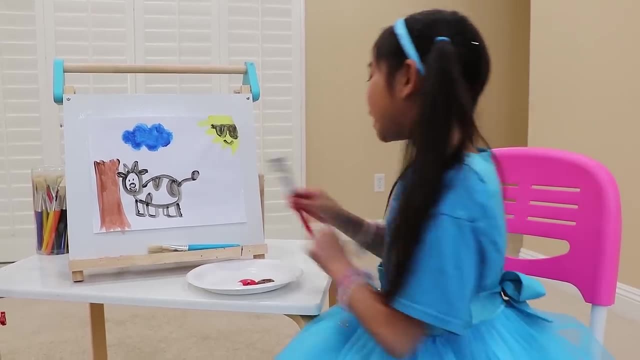 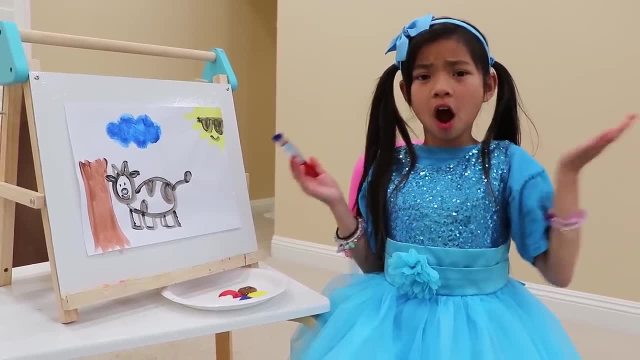 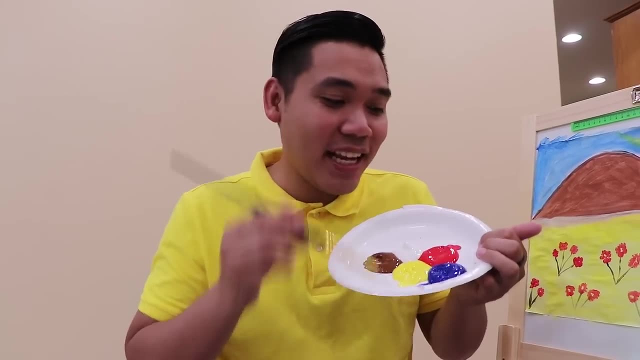 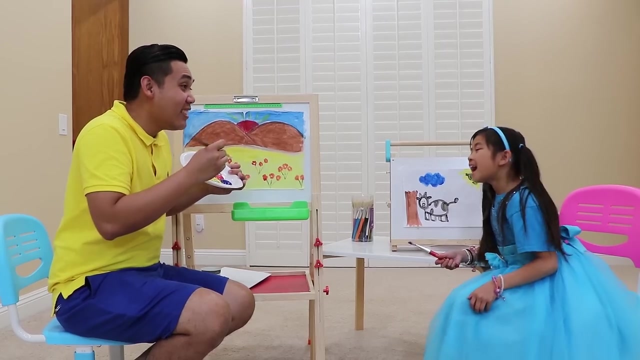 Really? Yeah, I'll show you, Thank you. You can make green by mixing yellow and blue. Let me show you. Look, I made green, I made green. See, it's turning green. Wow, Yeah, you can make more colors. 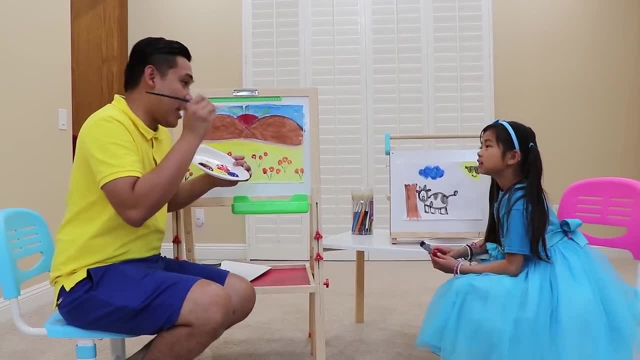 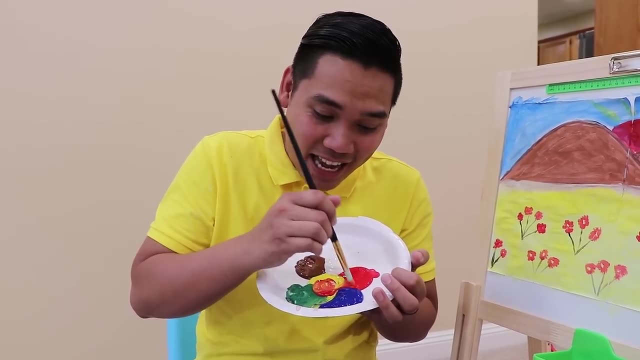 If you mix yellow and red, you will get orange, And if you want to make purple, you can mix red and blue. Let me show you. See, it turned to orange, guys, And now it will turn to purple. Thank you, Uncle John. 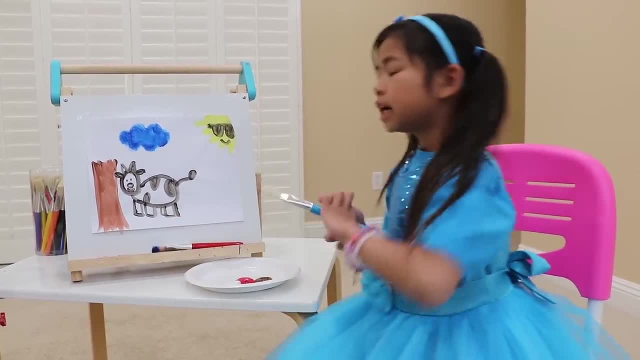 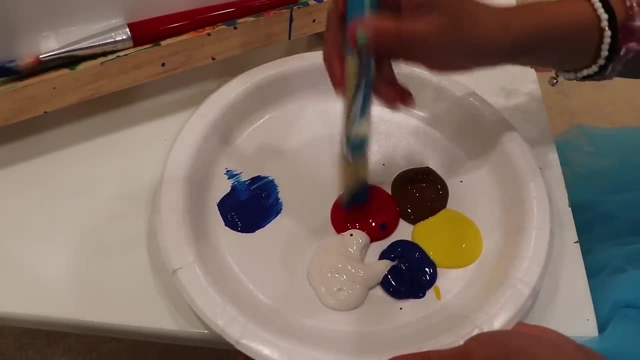 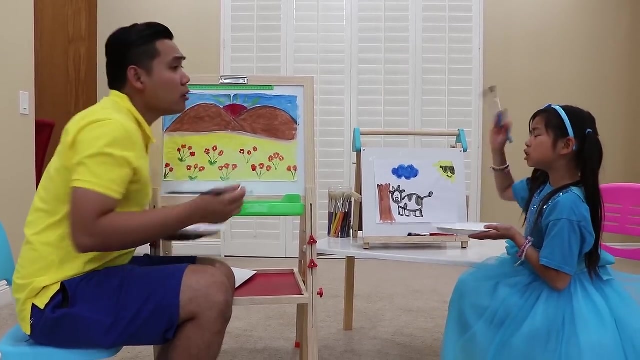 Let me try. I think blue and red make green guys. Let's try it. Let's do blue and red. Huh, It's purple guys, Uncle John. Uncle John, Huh, What happened, Emma? There are too many colors to mix and I don't remember what to make green? 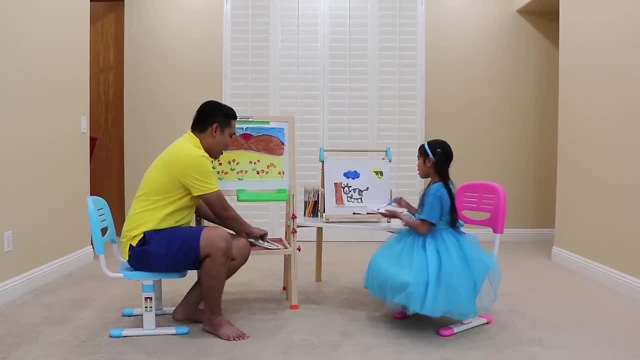 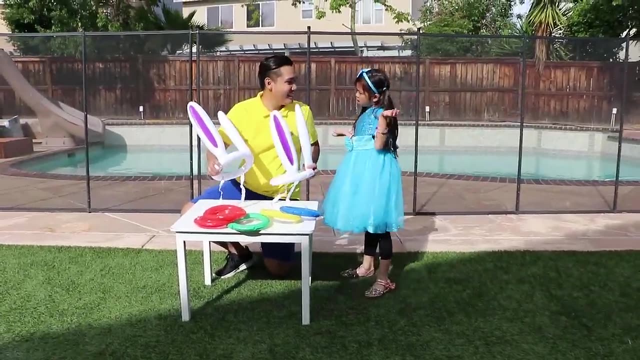 Really. Yeah, Don't worry, Follow me, I'll show you. Let's go. I got this, Emma. Look. Huh, What is that for Uncle? I'll show you. Wear the hat first. Okay, This is a magical hat. 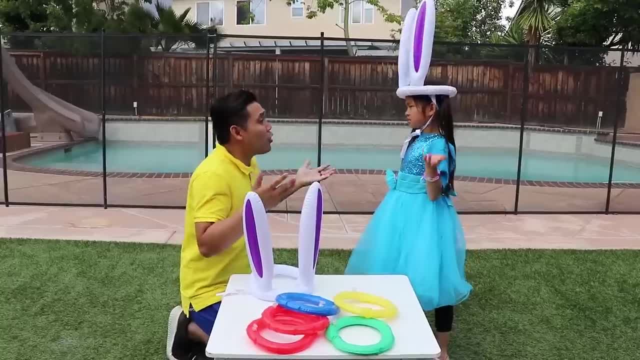 I'm done, Uncle John. What should I do next? Let me show you, Emma. Look, I have blue and yellow. Wow, I'm green. now Can I try it on you, Uncle? Yeah, Let me wear it. 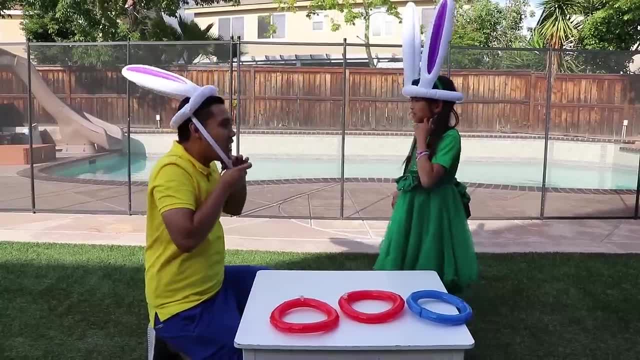 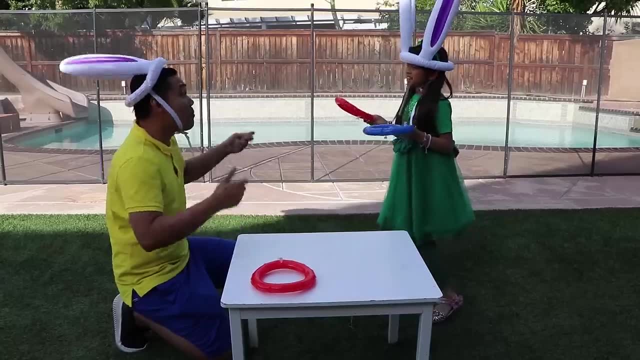 What color do you want to try? Hmm, I think I'll make purple. I need to use red and blue. Wow, Amazing, Try it, Emma. Okay, Wow, I'm wearing purple now. Yeah, I did it, Uncle John. 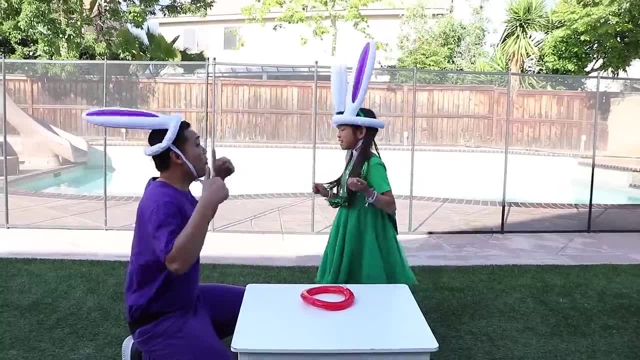 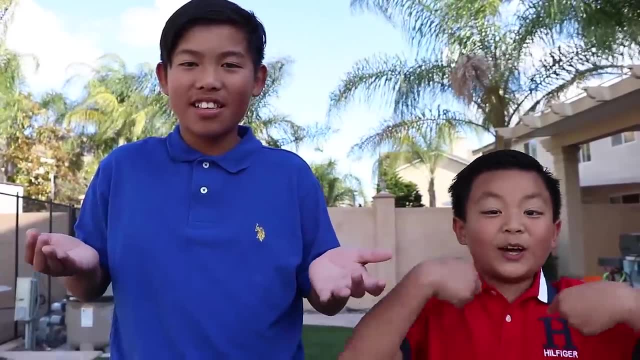 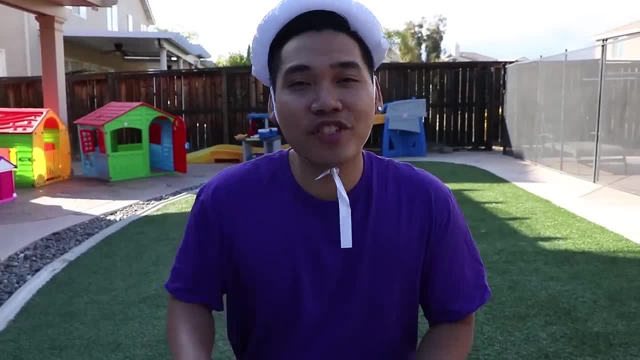 Uncle Emma, what are you doing? Can we play too? We're learning how to mix colors. Huh, How do you do that? Let me show you. If you want to make orange, you can make red and yellow, Huh. 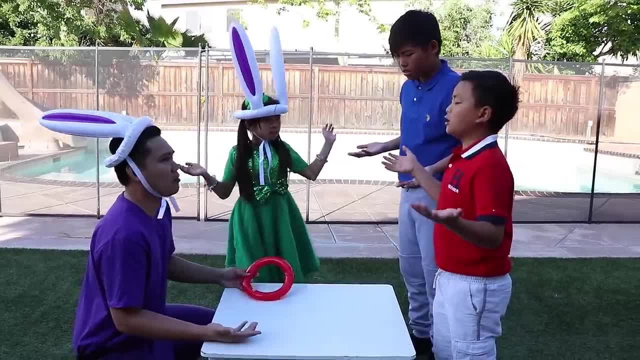 What happened, Uncle John? We have no more colorful ring to play with. Huh, We can't play. We're so sad. Hmm, Ah, I got an idea. I will go to the store and buy more ring for you. 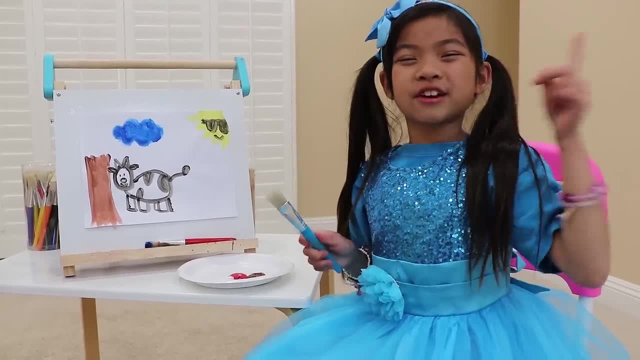 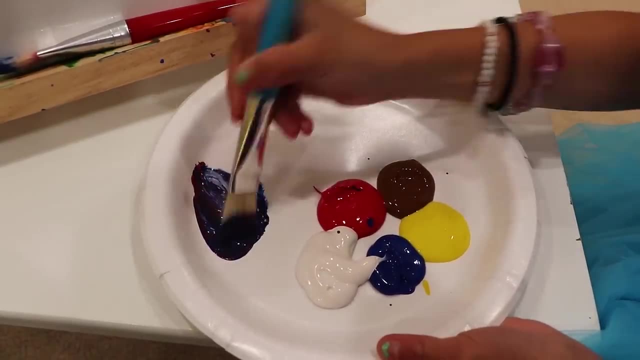 Hmm, I think blue and red make green guys. Let's try it, Let's do blue. Let's do blue and red. Huh, It's purple guys. Uncle John, Uncle John, Huh, What happened, Emma? 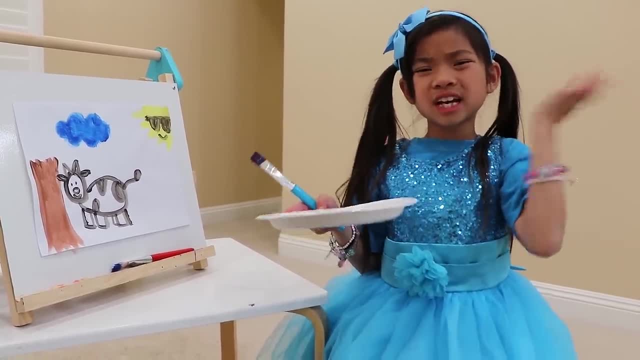 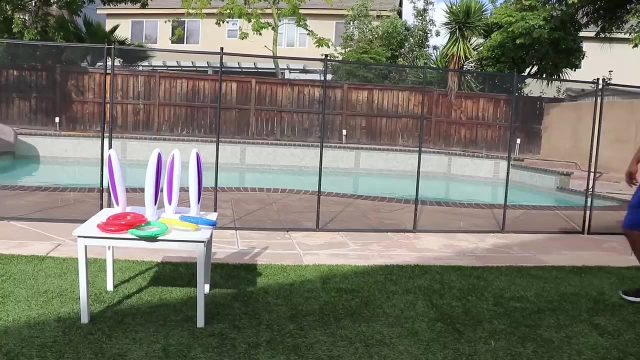 There's too many colors to mix and I don't remember what to make. green, Hmm, Really. Yeah, Don't worry, Follow me, I'll show you. Let's go. I got this, Emma, Look, Huh. 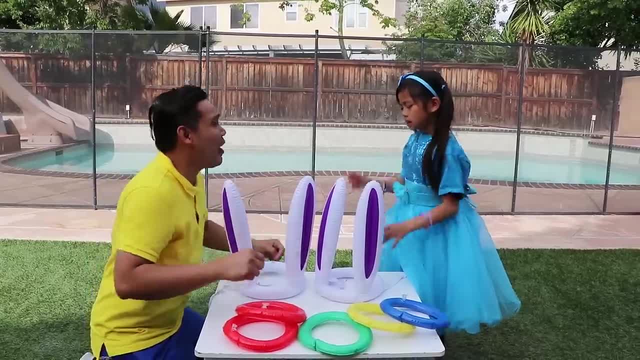 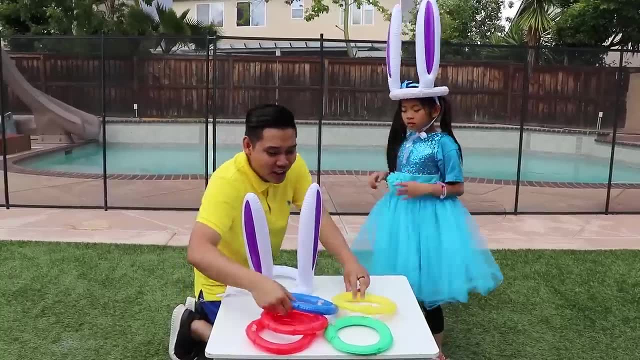 What is that for Uncle? I'll show you. Wear the hat first. Okay, This is a magical hat. I'm done, Uncle John. What should I do next? Let me show you. Emma, Look, I have blue and yellow. 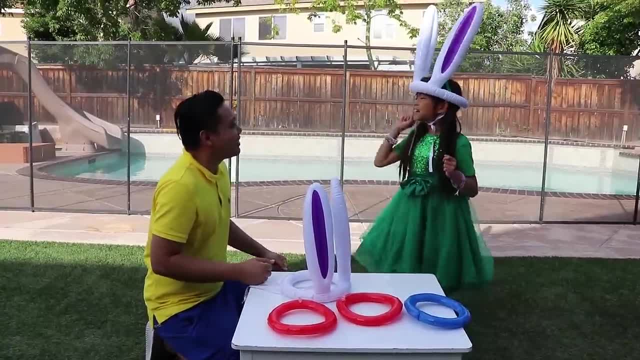 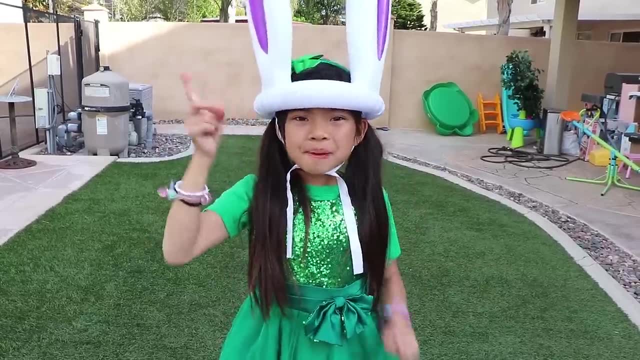 Wow, I'm green. now Can I try it on you, Uncle? Yeah, Let me wear it. What color do you want to try? Hmm, I think I'll make purple. I need to use red and blue. Wow, Amazing, Try it, Emma. 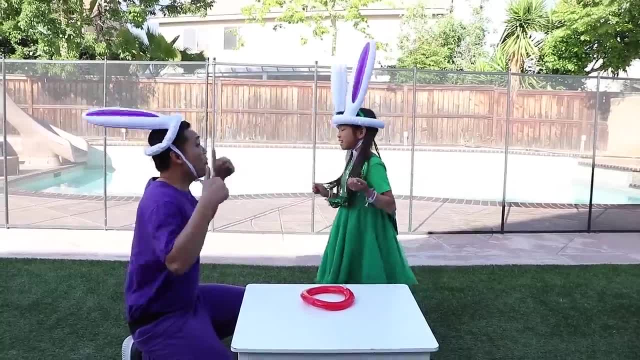 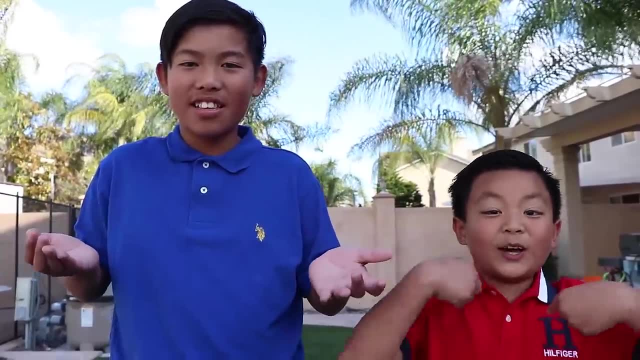 Okay, Wow, I'm wearing purple now. Yeah, I did it, Uncle John. Yay, Uncle Emma, what are you doing? Can we play too? We're learning how to mix colors. Huh, How do you do that? 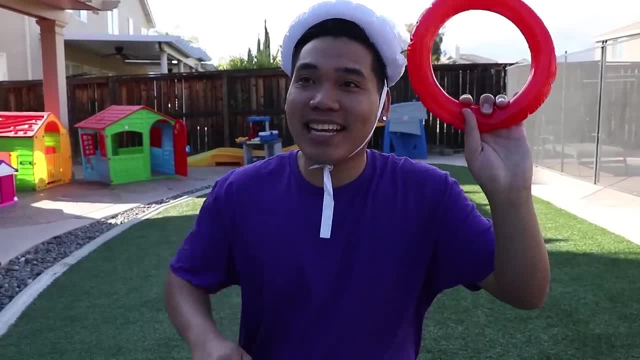 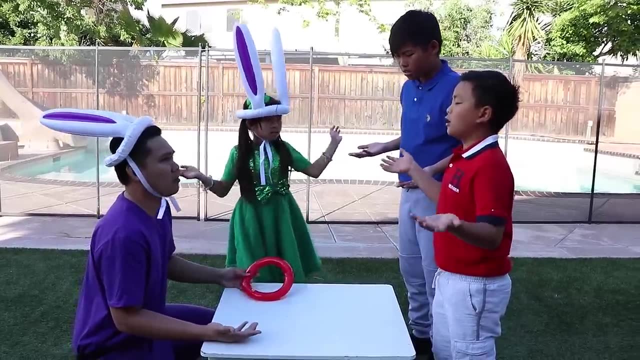 Let me show you. If you want to make orange, you can mix red and yellow. Huh, What happened, Uncle John? We have no more colorful ring to play with. Huh, We can't play. We're so sad. 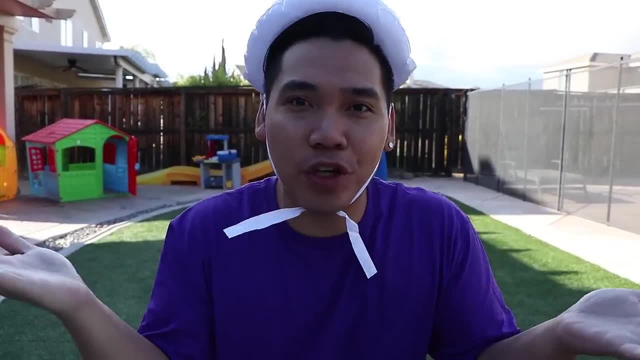 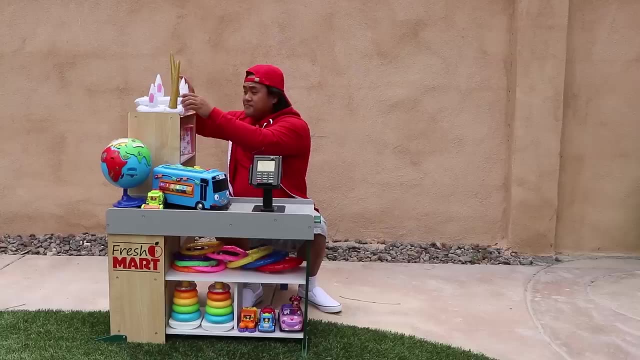 Ah, I got an idea. I will go to the store and buy more rings for you. Really, Uncle John? Yeah, Can you teach them how to play? I'll come back with a ring. Okay, Bye guys. Hi, Uncle Sam, Hi, Uncle John. 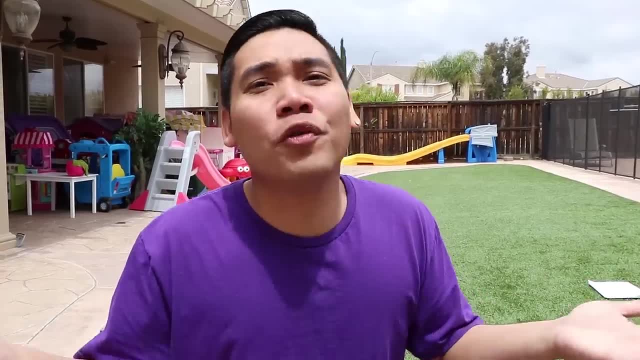 Welcome to my store. How can I help you? today I want to buy the colorful rings for Emma. Colorful rings- Yeah, Oh, I have one right here, Check it. Hmm, I don't want that ring, Uncle Sam. 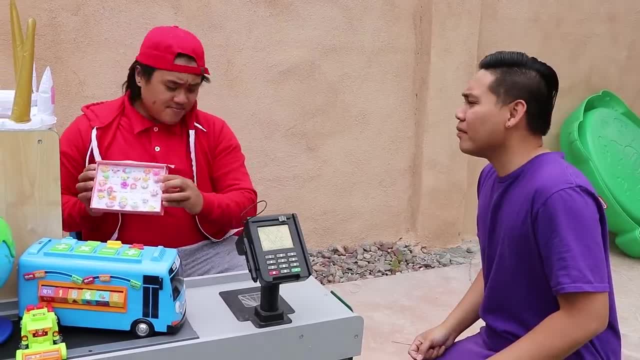 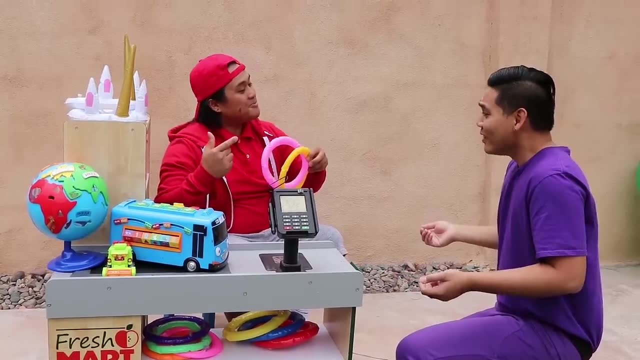 I want the ring for the ring toss, Ring toss. Yeah, Oh, We have one right here. Check it out. Hmm, Yeah, That's the one. How much is it? Only $2,, please, $2?. Here's your money, Thank you. 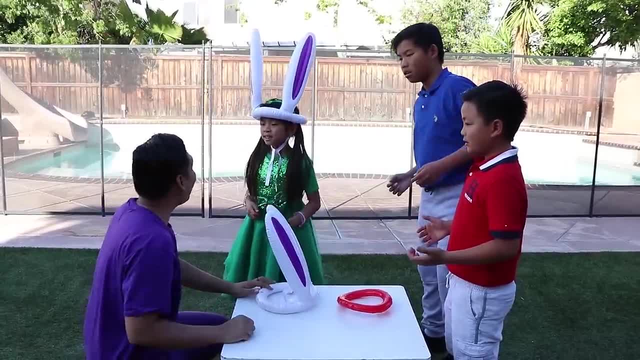 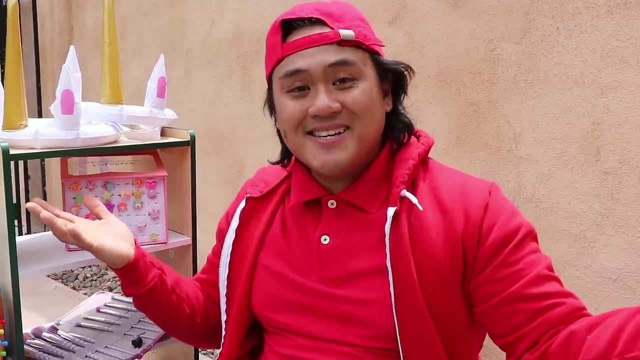 Really, Uncle John. Yeah, Can you teach them how to play? I'll come back with a ring. Okay, Hi, Uncle Sam, Hi, Uncle John, Welcome to my store. how can I help you? today, I want to buy the colorful rings for Emma. 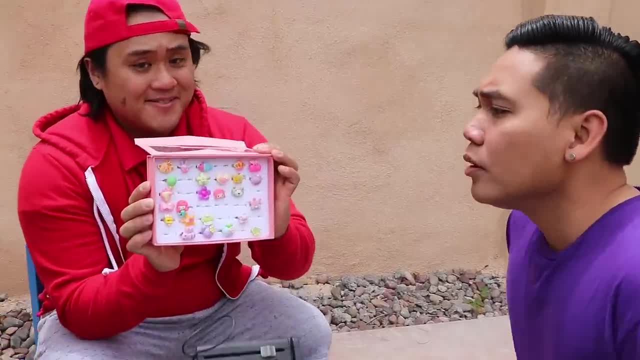 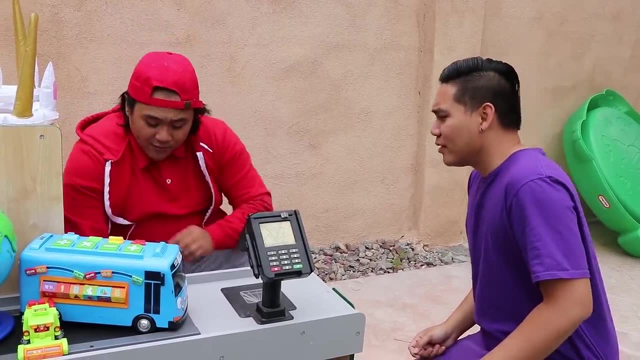 Colorful rings. Yeah, Oh, I have one right here, check it. Hmm, I don't want that ring, Uncle Sam, I want the ring for the ring toss, Ring toss. Yeah, Oh, we have one right here, check it out. Hmm, Yeah, that's the one. how much is it? 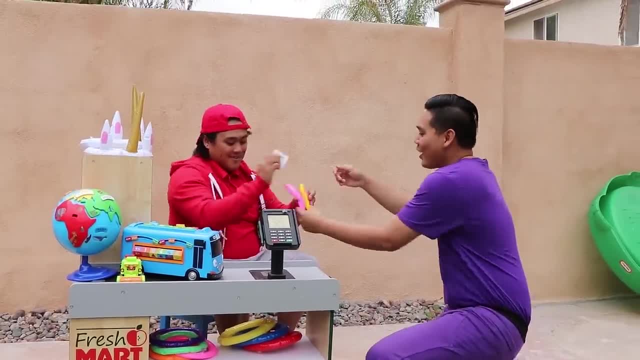 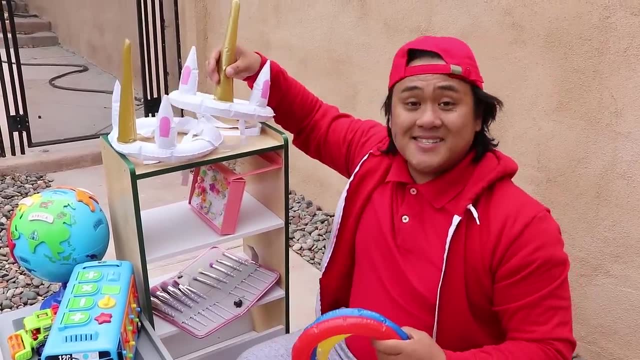 Only 2 dollars. please 2 dollars, Here's your money. Thank you, Wait, Uncle John. Huh, What happened? Uncle Sam, We have a special deal today: If you buy all these rings, you get these hats. Wow, that's a really good deal. 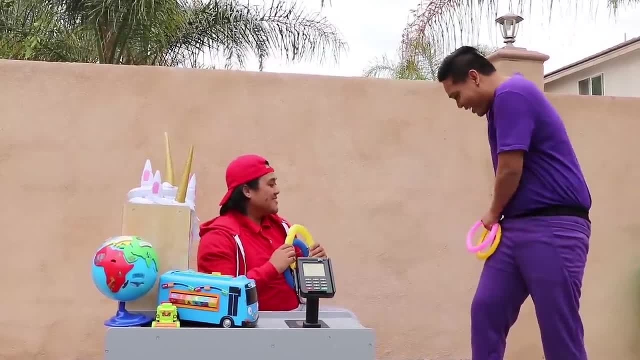 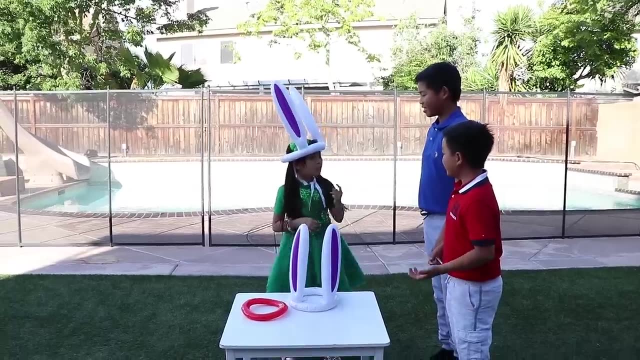 I will get everything. How much is it? Another 2 dollars, please. Okay, Here you go, Thank you. Thank you, Here you go. Wow, thank you, bye, Bye. Yellow and blue makes green guys. Wow, Thank you, Emma. Hey guys, look at this. 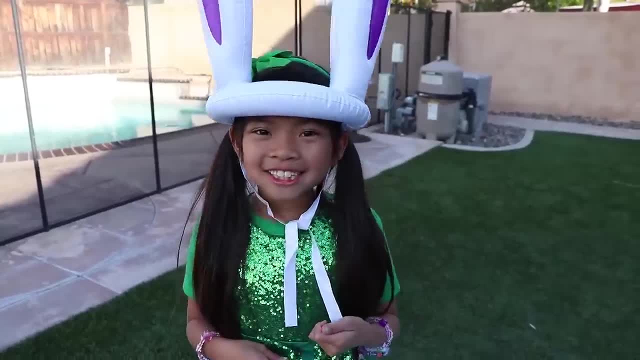 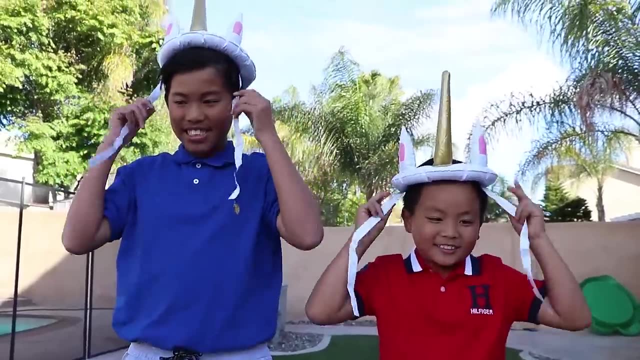 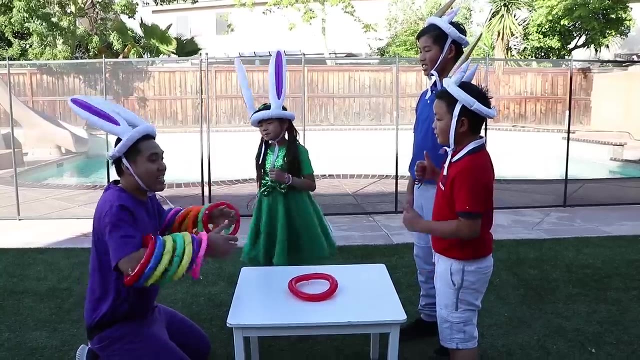 Wow, Thank you, Uncle John. No problem, Emma, I have this hat for Alex and Michael. Wow, thank you, Uncle John. Thank you, Uncle John. Here you go, And since we have a lot of rings, let's do a competition. Cool, but these are the magical rings. 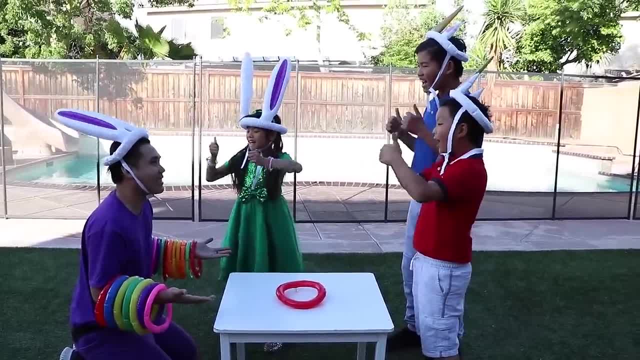 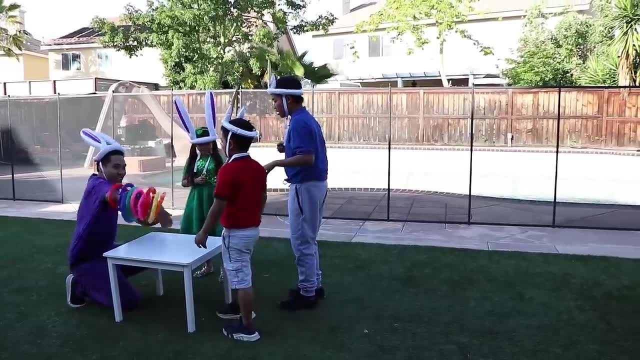 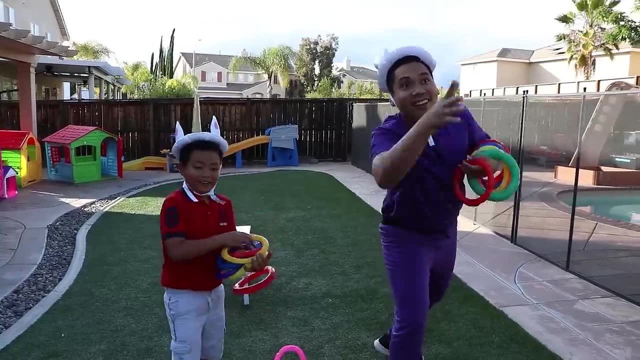 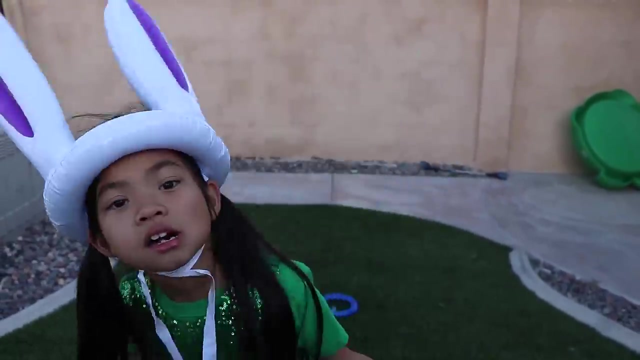 So you have to two of them in one at a time. okay, Okay, Ready guys, Set go. Yay, Let's play Uncle. Okay, here you go, Let's play. Hmm, Huh, Huh, Huh, Oh no, we're losing. 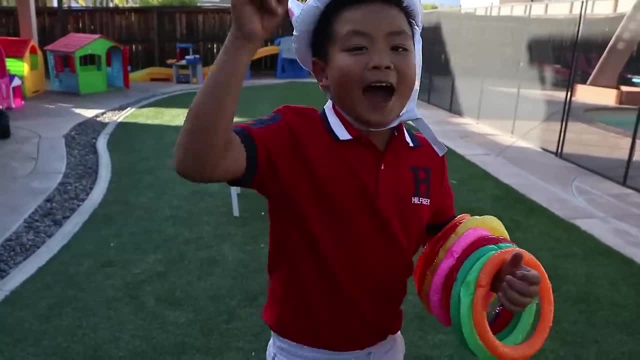 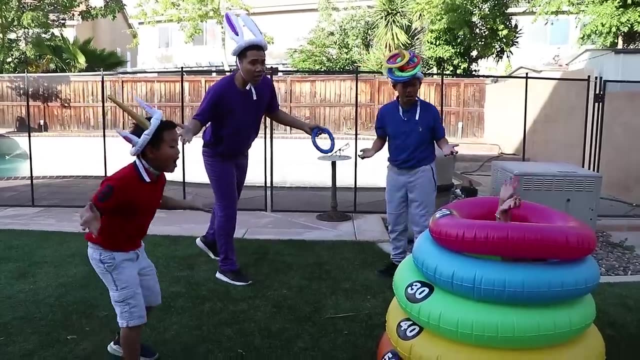 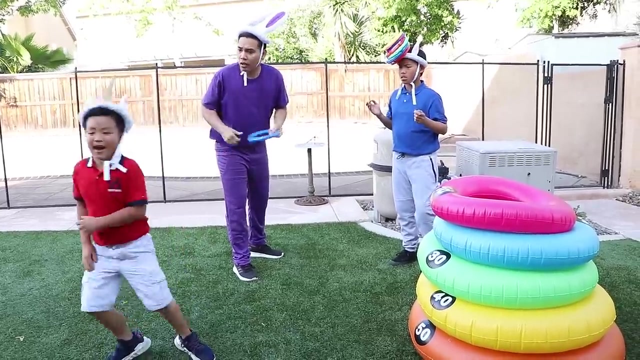 I have an idea. I'm going to throw it all at once. Yeah, we won. Oh no, the ring buzzer changed to make Emma stop. What should we do? I have an idea. Wait here, I'll be right back. Okay, Don't worry, Emma, we'll save you. 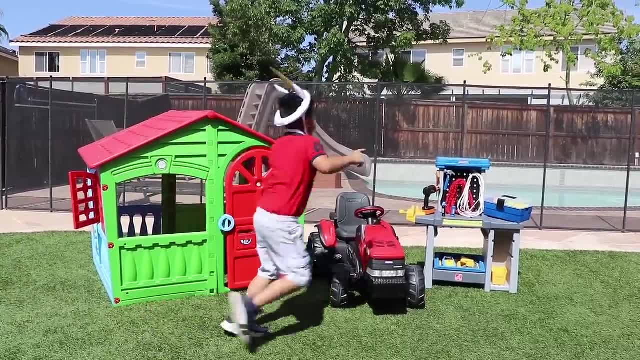 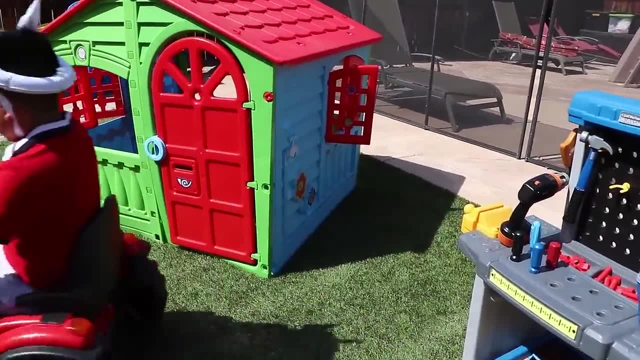 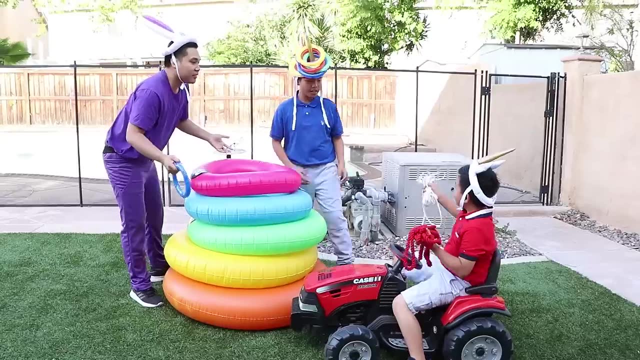 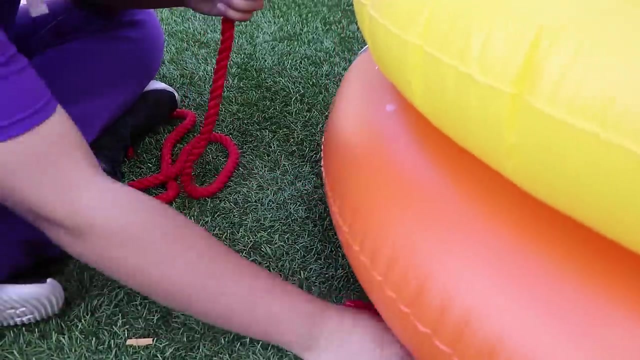 Hmm, There it is, Let's go guys. Don't worry, Emma, we will help you. Here it is. Let's tie these ropes to the ring Here. let me help you. Okay, here, Here you go, Uncle John. Okay, Emma, catch Uncle, can you tie it for me? 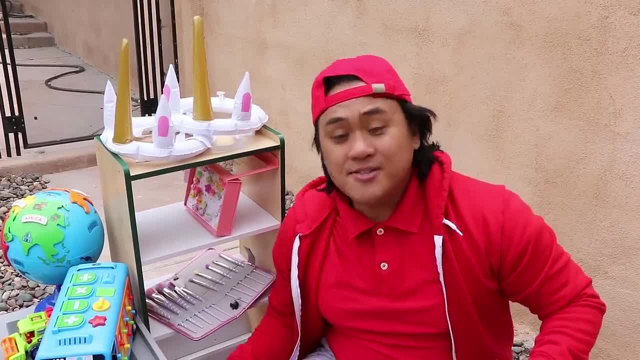 Wait, Uncle John. Huh, What happened? Uncle Sam, We have a special deal today. If you buy all these rings, you get these hats. Wow, That's a really good deal. I will get everything. How much is it? 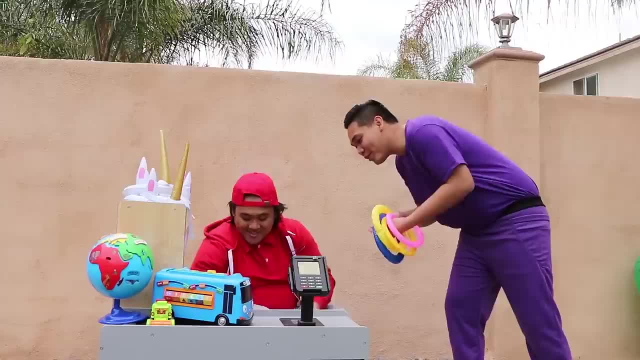 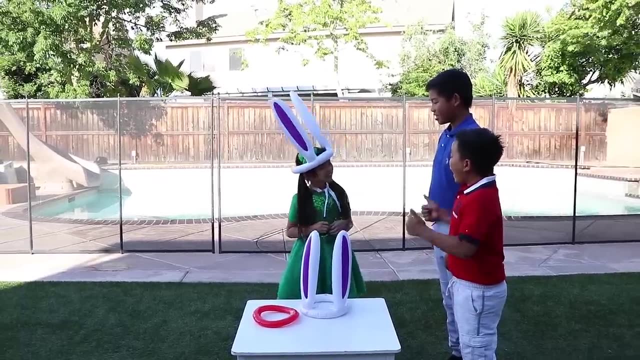 Another $2, please. Okay, Here you go. Thank you, Here you go. Wow, Thank you, Bye, Bye. Yellow and blue makes green guys. Wow, Thank you, Emma. Hey guys, Look at this. 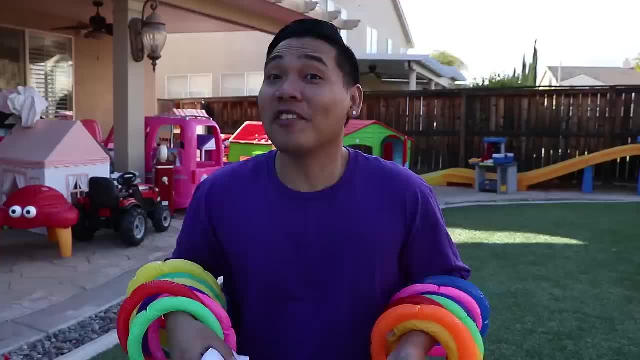 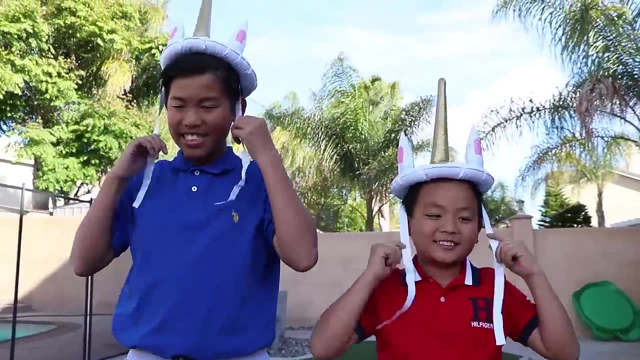 Wow, Thank you, Uncle John. No problem, Emma, I have this hat for Alex and Michael. Wow, Thank you, Uncle John. Here you go. And since we have a lot of rings, let's do a competition. And since we have a lot of rings, let's do a competition. 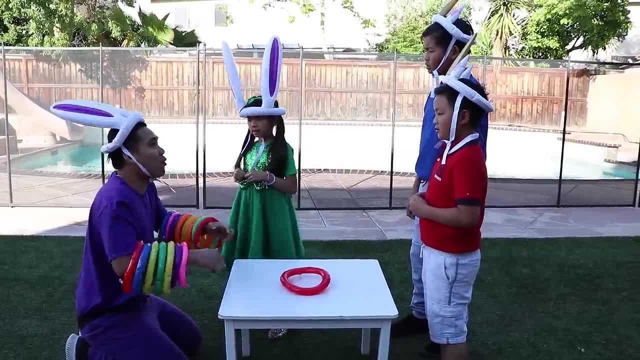 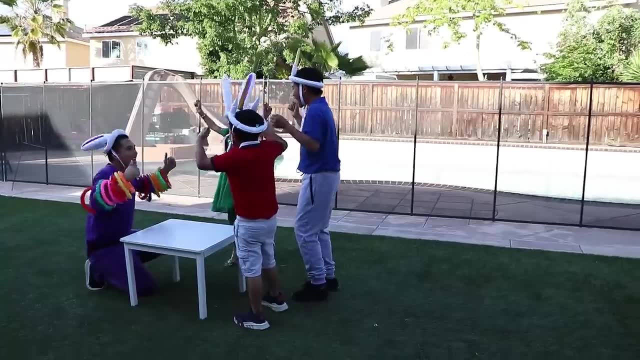 Cool, But these are the magical rings, so you have to throw them in one at a time. okay, Okay, Ready guys, Set go. Yay, Let's play, Uncle. Okay, Here you go, Let's play. 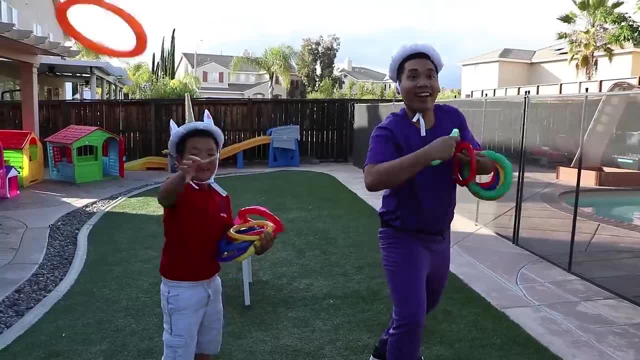 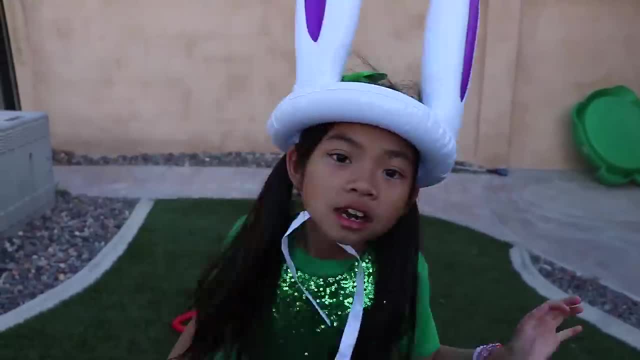 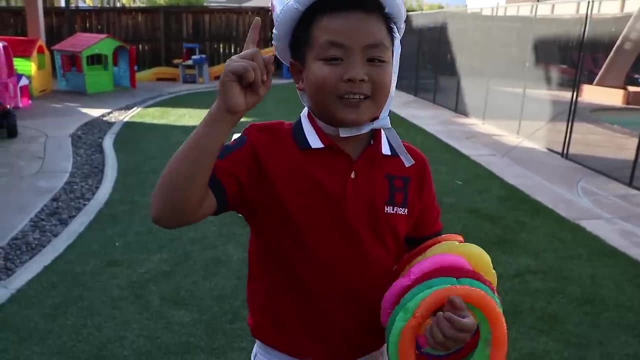 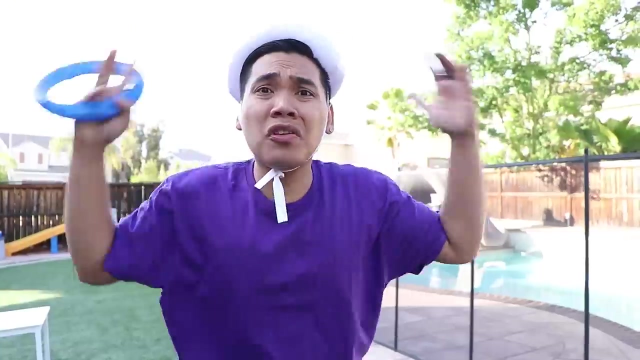 Hmm, Huh, Huh, Hmm. I have an idea. I'm going to throw it all out at once. yeah, we won. oh no, the ring buzzer changed to make Emma stop. what should we do? I have an idea. wait here, I'll be. 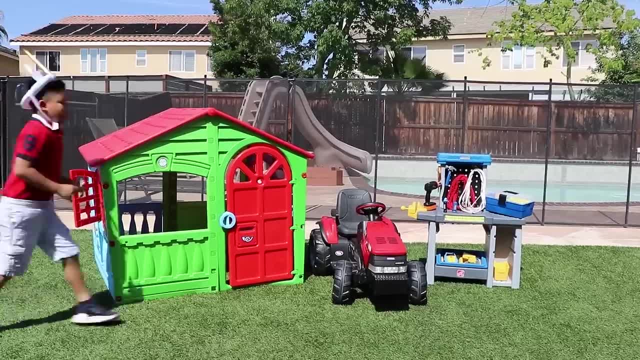 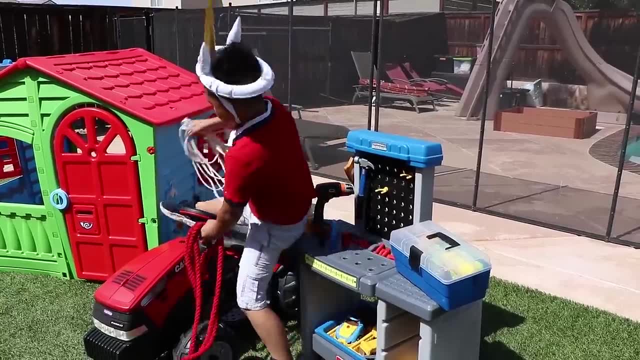 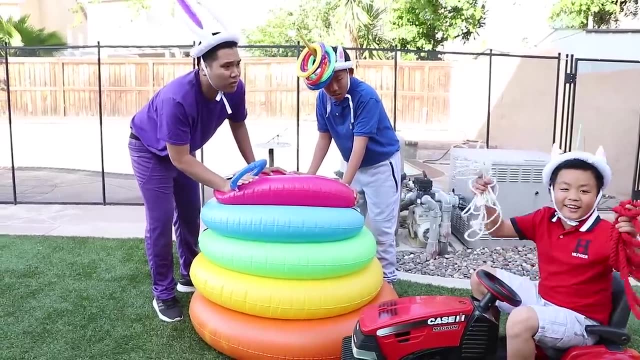 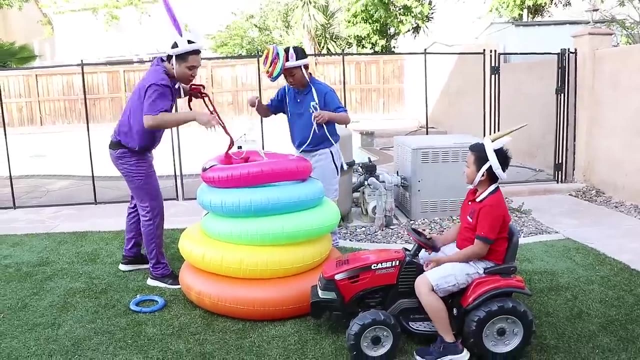 right back. okay, don't worry, Emma, we'll save you. there it is, let's go guys. don't worry, Emma, we will help you. here it is, let's tie these ropes to the ring here. let me help you. okay, here, here you go, Uncle John. okay, Emma, catch Uncle, can you tie? 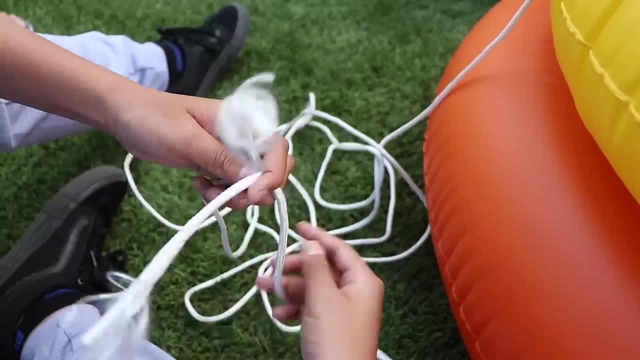 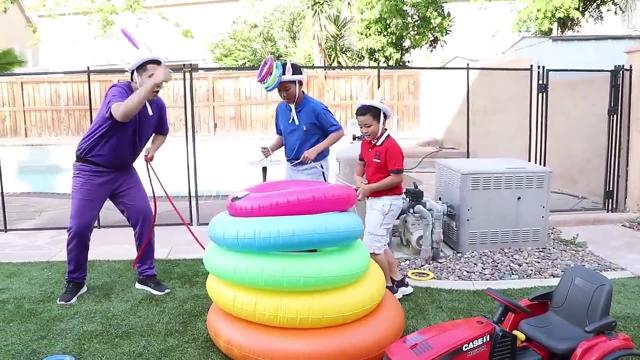 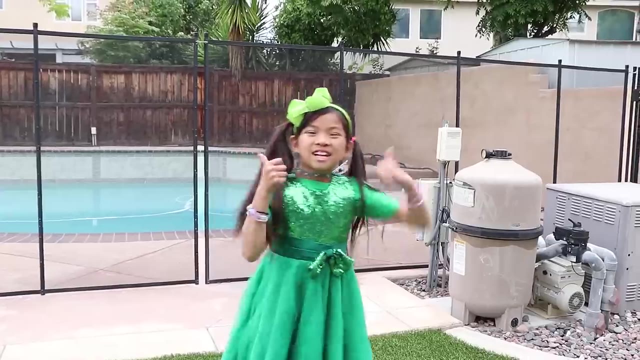 it for me. okay, Alex, can you help me? yeah, are you ready guys? yeah, okay, 1,, 2,, 3,, 4, yeah, I'm free. yeah, thank you for saving me everyone. no problem, Emma, remember to help each other. 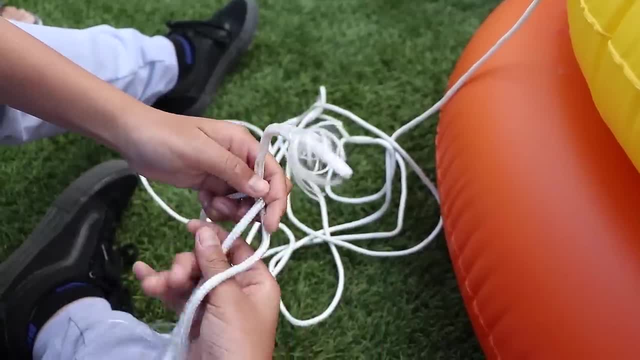 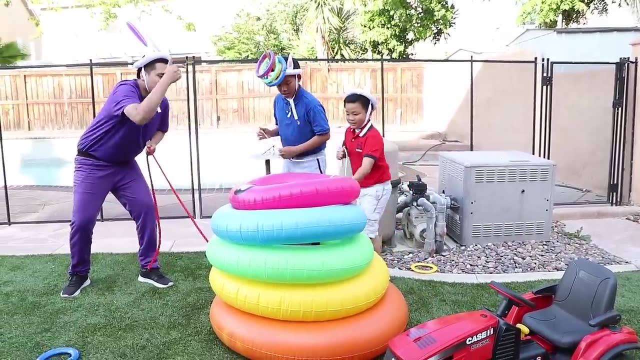 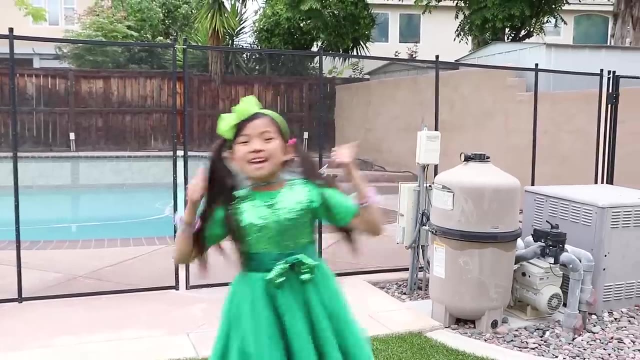 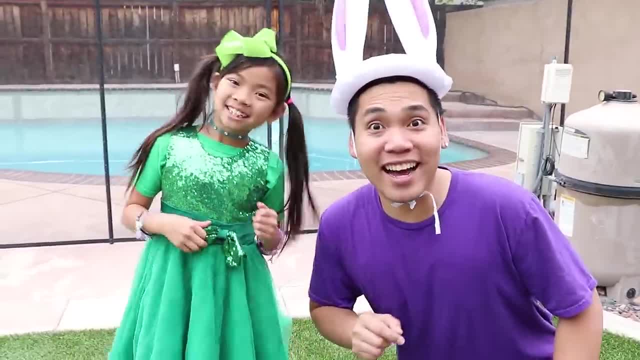 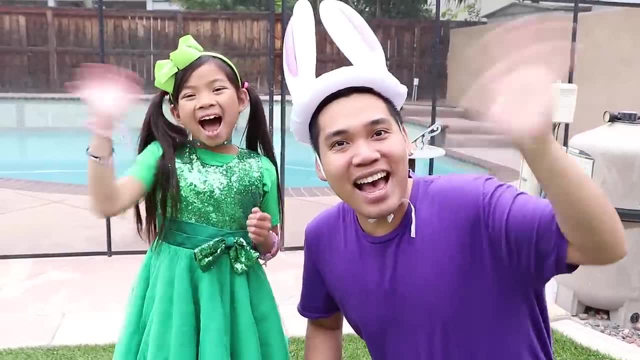 No problem, Emma, Remember to help each other guys. Thank you for watching. Hope you guys enjoy our show. Please remember to subscribe to our channel. Click the bell button. See you next time. Bye, Ooh, that would be so cool. Let me try to read it. 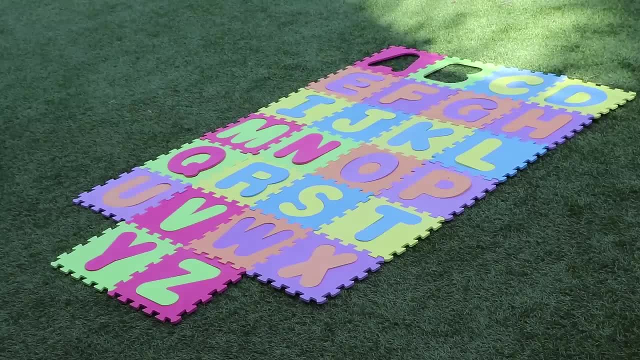 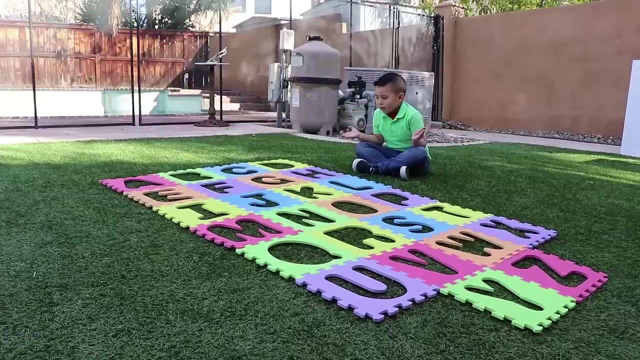 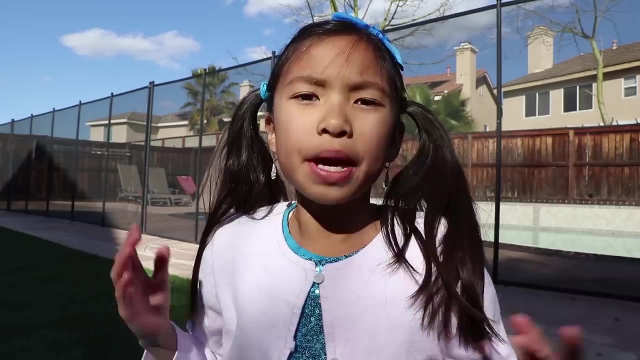 S-G-B. See H-I-J-K-L-M-N-I. Huh, That one bit disappeared. What should I do? Huh, What happened, Liam? The letters disappeared Wednesday. Maybe you read it wrong, So that's why they disappeared. Let's go find them, Liam. 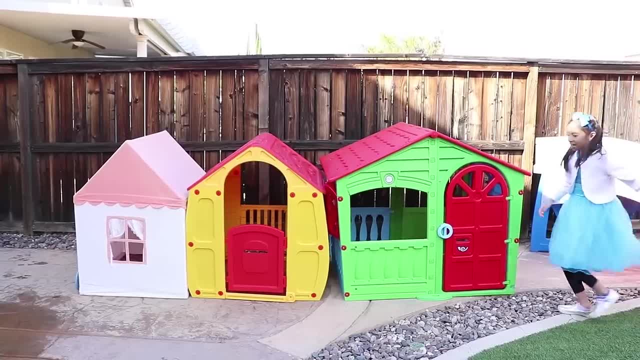 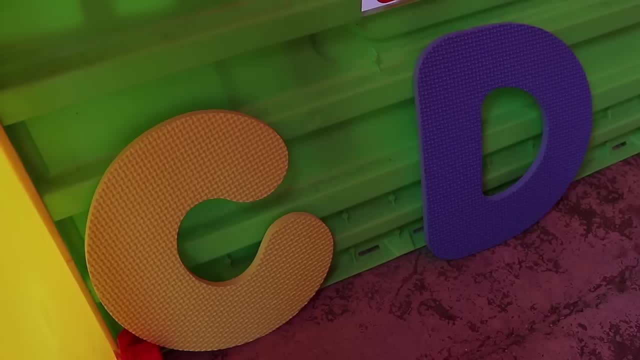 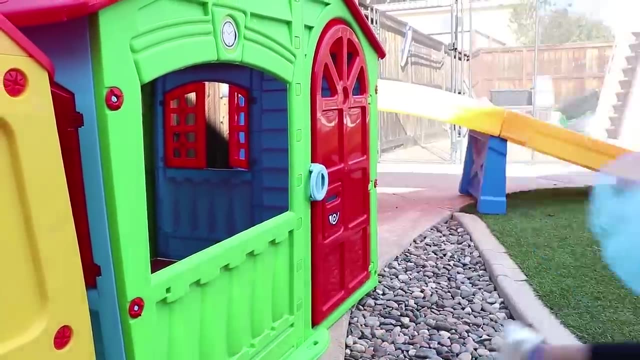 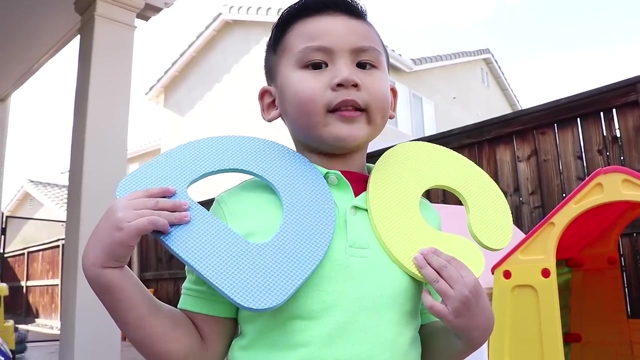 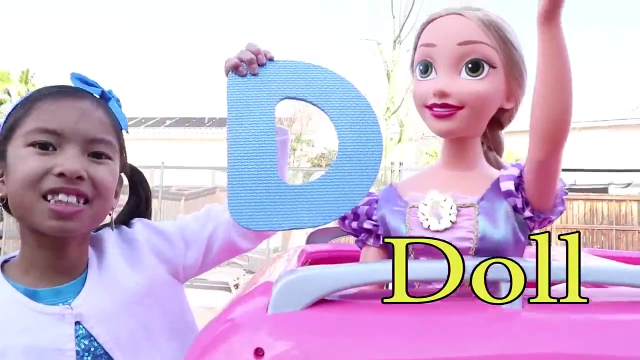 Okay, Let's look for letters. Okay, Wow, I found A And B. Where are these letters? Let me show you: Liam, A is for apple And B is for ball. Cool, Where are these letters? Wendy, C is for car And D is for doll. I got that, Wendy. 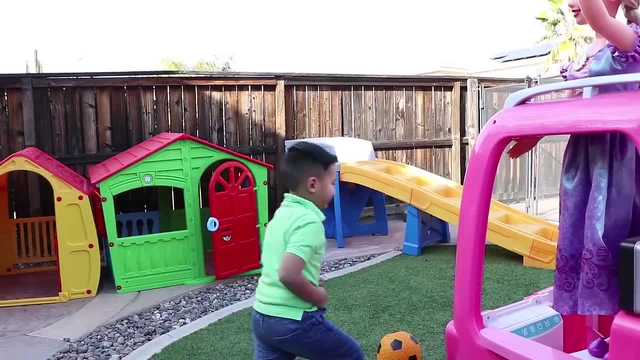 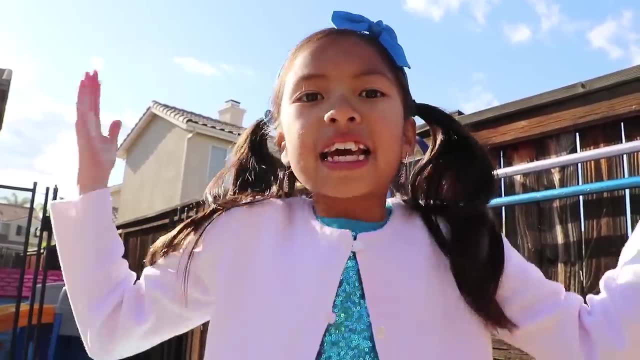 Let's go find more letters, Liam. Okay, Hi, Uncle John, Hi guys, Hi, What are you guys doing here? We are looking for letters. Can you help us? Okay, let me help you, Let's go. Let's go, Liam, Let's go Liam. 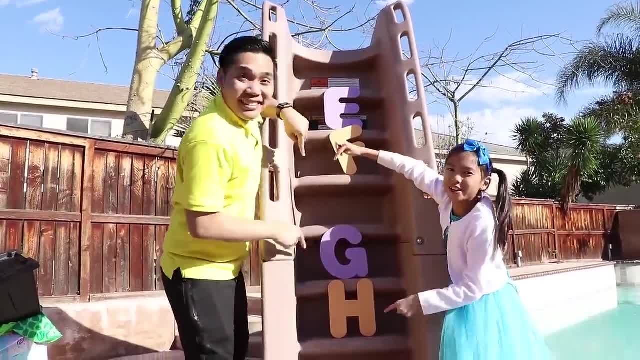 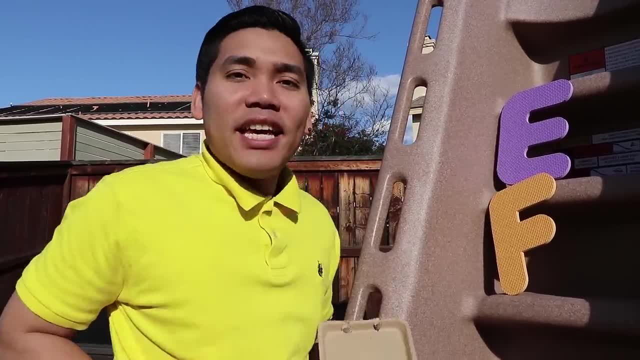 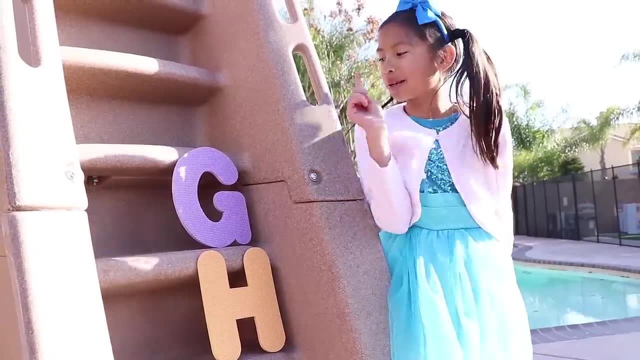 Ah, I found some letters here And I found these too Cool. Where are these letters? That's very easy, Liam. Let me show you. This is letter E- E for the egg. And this is letter F- F for flower. And look, Liam, G is for guitar. 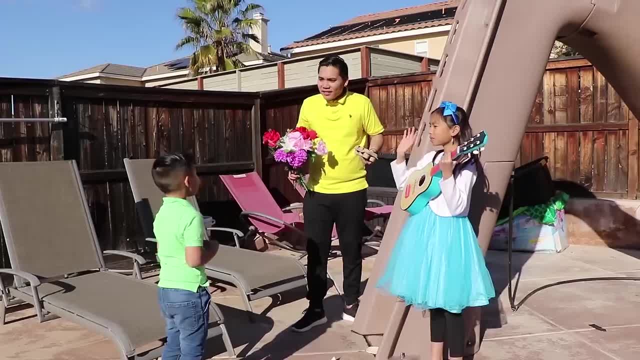 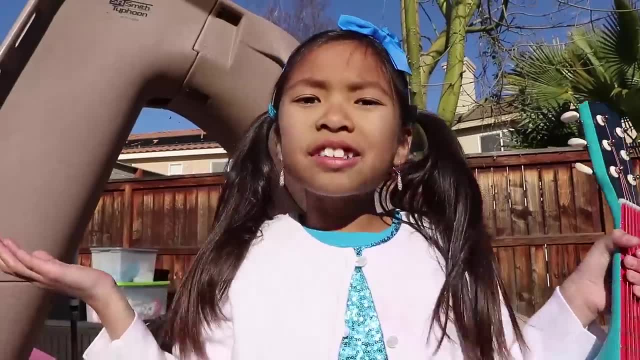 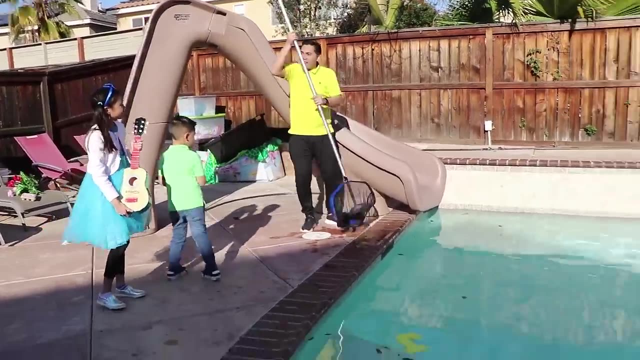 Y and H is for hand Boy. I got it. Oh guys, Look, I see some letters here. Uncle, how can we get them? They're in the pool. Don't worry guys, Look at me, I will use this to catch them. Check it out, guys. 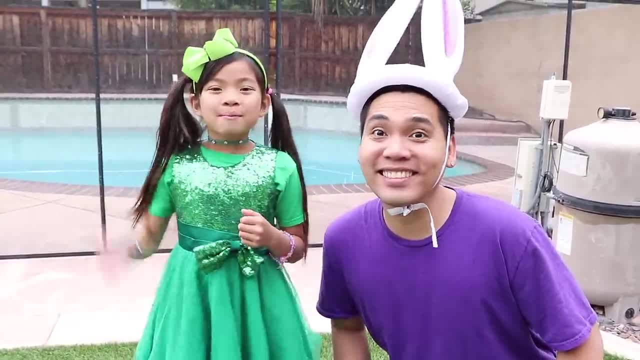 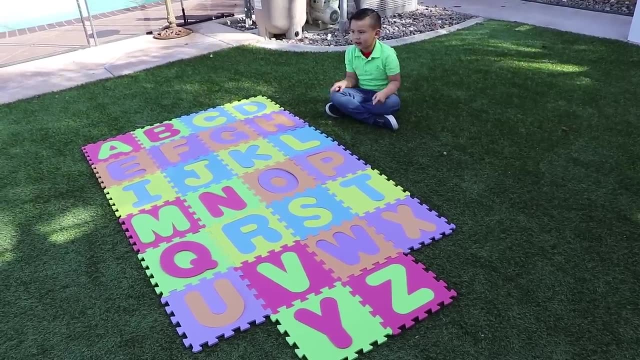 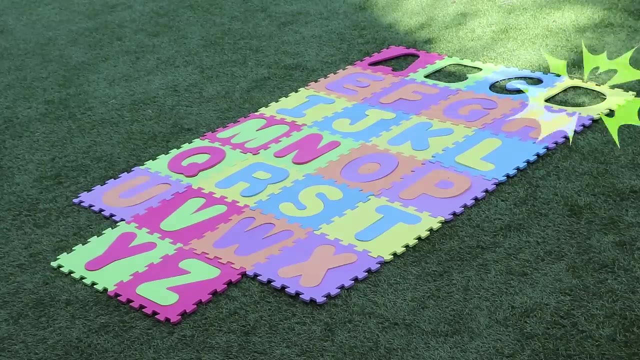 guys. thank you for watching. hope you guys enjoy our show. please remember to subscribe to our channel. click the bell button. see you next time. bye, so cool. let me try to read it: S, G, P, C, H, I, J, K, L, M, N, H, that one bit. 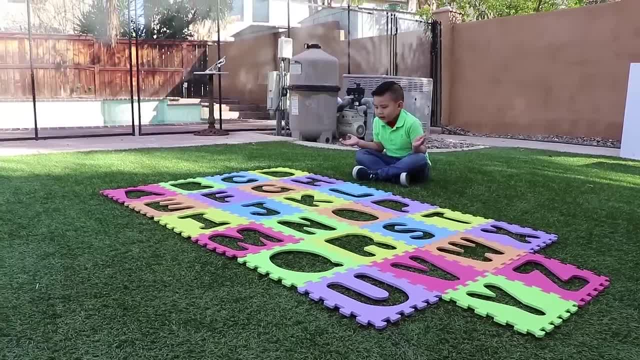 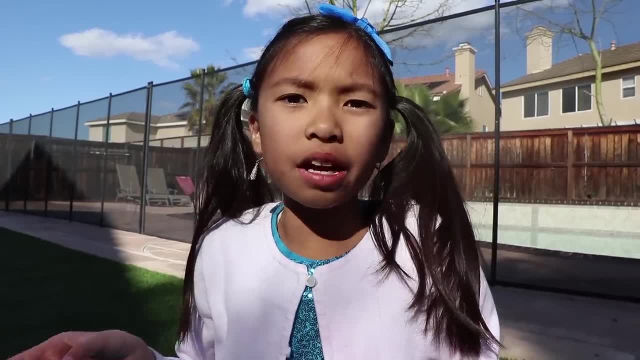 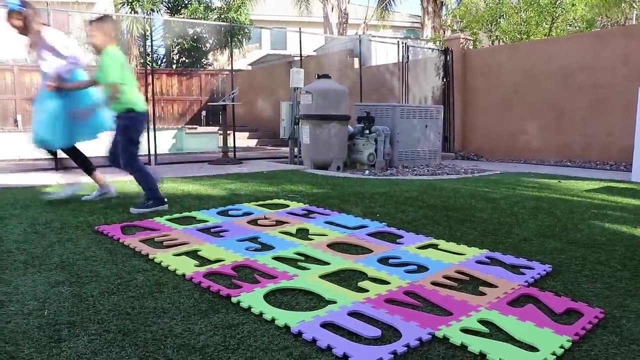 disappeared. what should I do? huh, what happened, Mia? the letter disappeared Wednesday. maybe you read it wrong, so that's why they disappeared. let's go find them, Mia, okay? A, B, C, D, E, F, G, H, I, J, K, L, M, N, H, I, J, K, L, M, N, H, I, J, K, L, M, N, H, I, J, K, L, M. 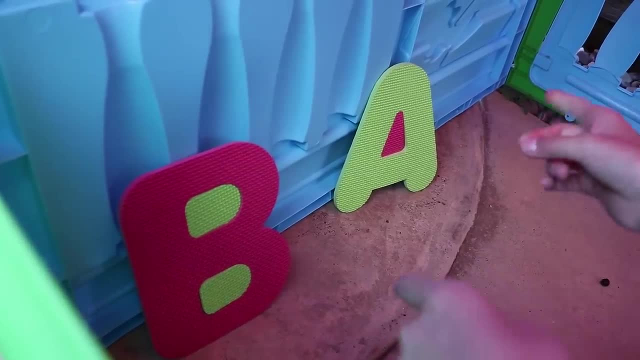 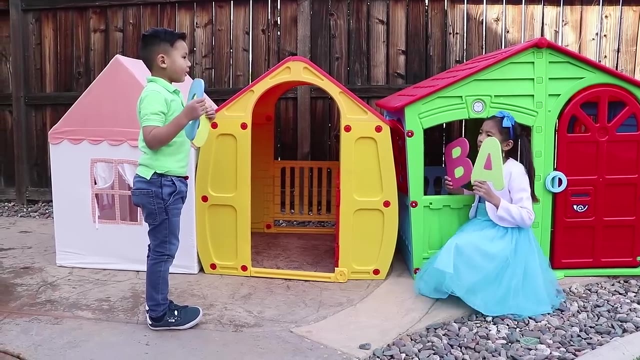 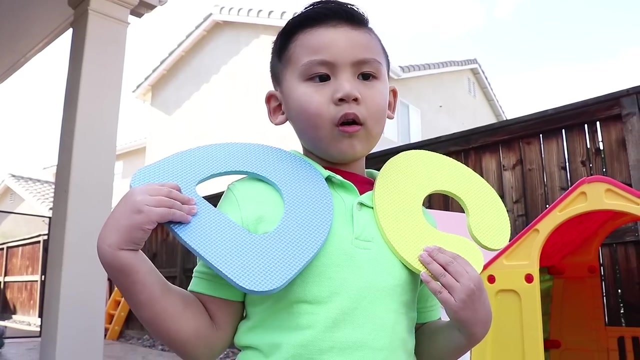 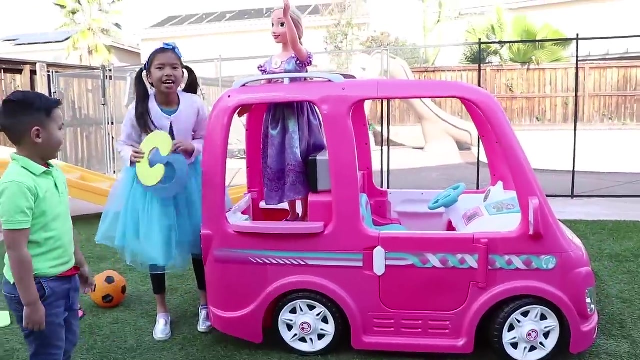 I found four letters. okay, wow, I found A and B. where are these letters? let me show you: A is for apple and B is for ball. cool, where are these letters, Wendy? C is for car and D is for doll. I got that, Wendy. let's go find more letters. wow, they are so big. 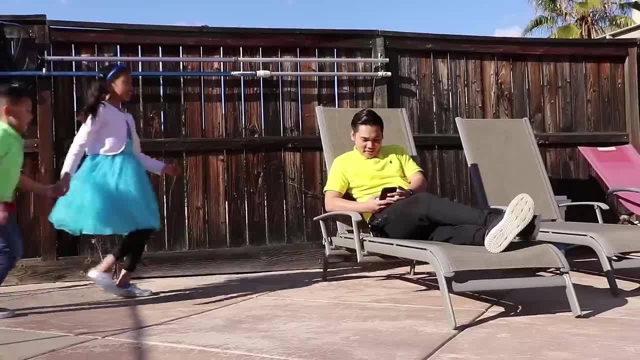 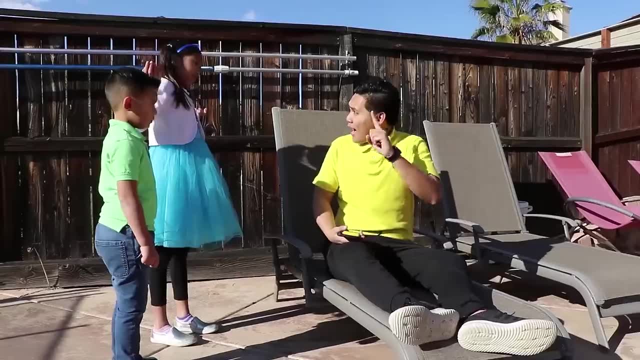 For letters, Liam. Okay, Hi, Uncle John, Hi guys, What are you guys doing here? We are looking for letters. Can you help us? Okay, let me help you. Let's go. Let's go, Liam. 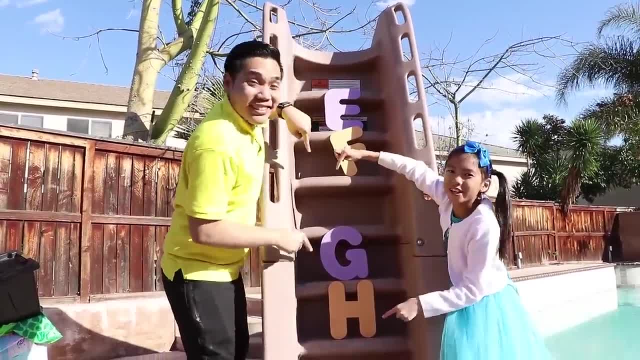 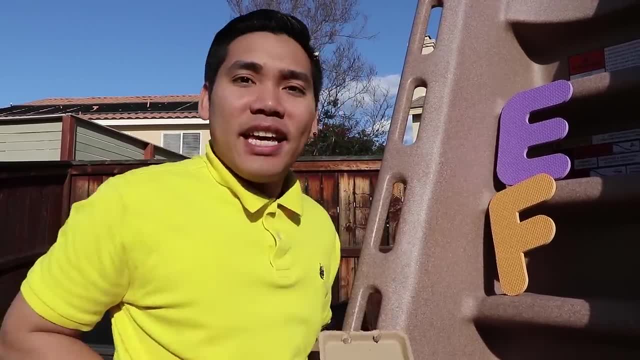 Ah, I found some letters here, And I found these too. Where are these letters? That's very easy, Liam. Let me show you. This is letter E- E for the X, And this is letter F- F for flower. 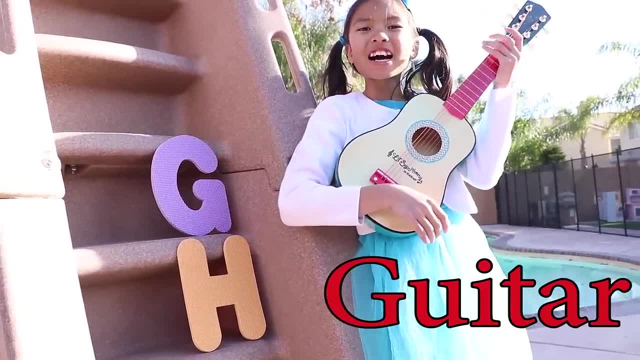 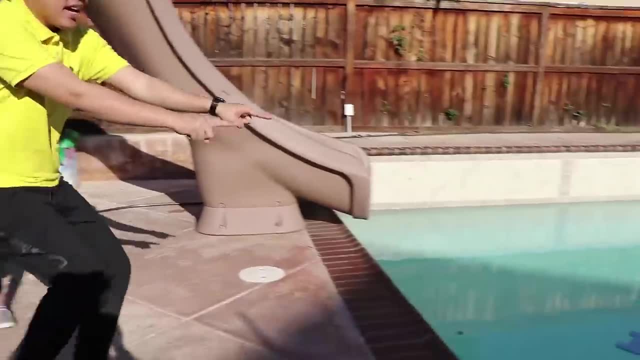 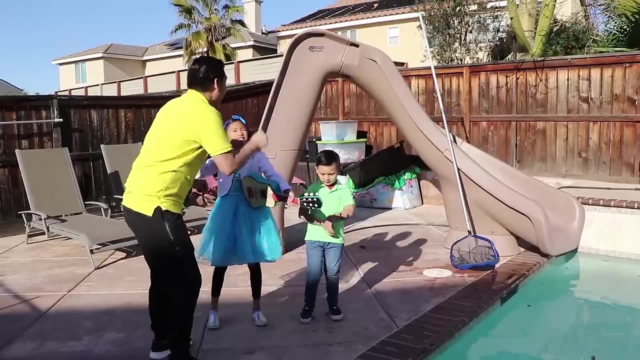 And look, Liam, G is for guitar And H is for hand. Oh, I got it. Oh guys, Look, I see some letters here. Uncle, how can we get them? They're in the pool, Don't worry, guys. 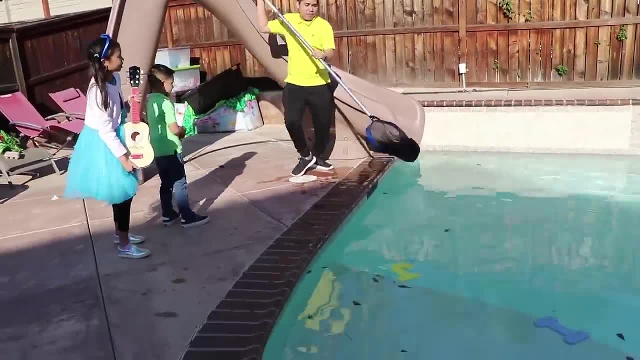 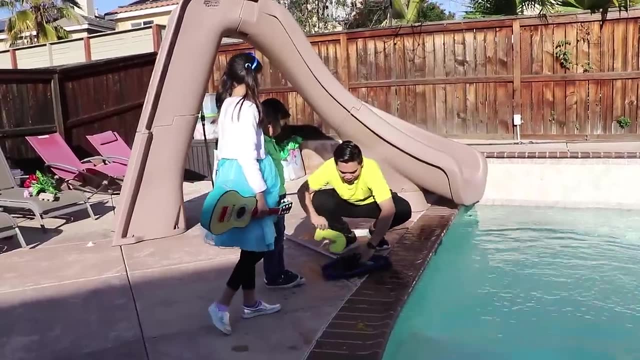 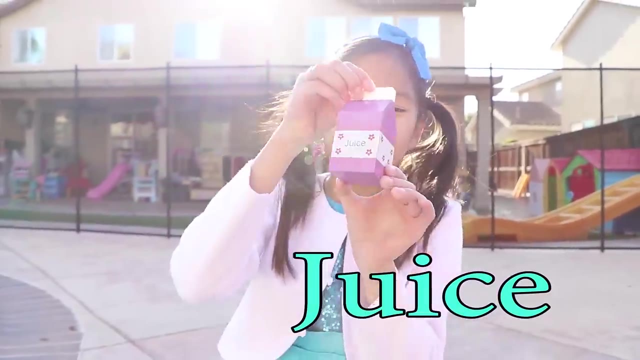 Look at me, I'll use this to catch them. Check it out, guys. I think I have letter J and letter I. Let me show you: Liam, I is for ice cream and J is for juice. Cool, I got it. 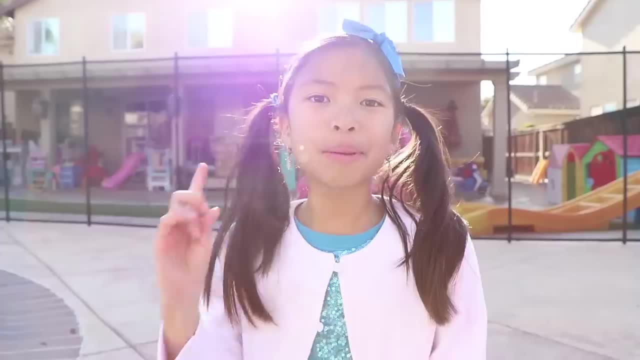 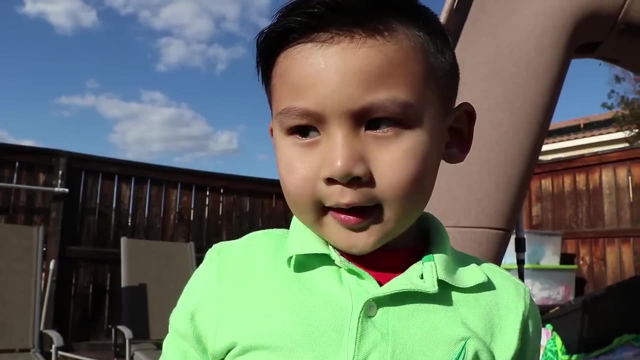 I think I have letter J And letter I. Let me show you: Liam, I is for apple, I is for ice cream And J is for juice. Cool, I got it. Let's go find more letters, Liam. Okay, Thank you, Uncle John. Bye, Bye, guys. 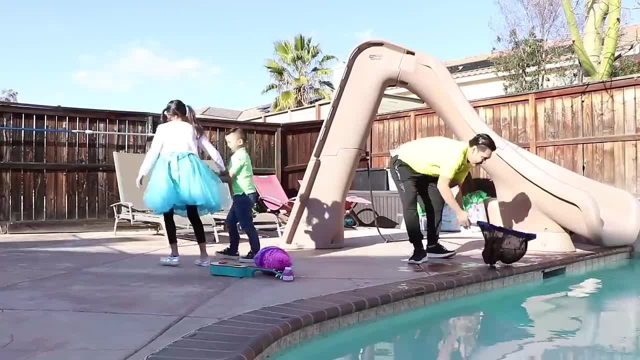 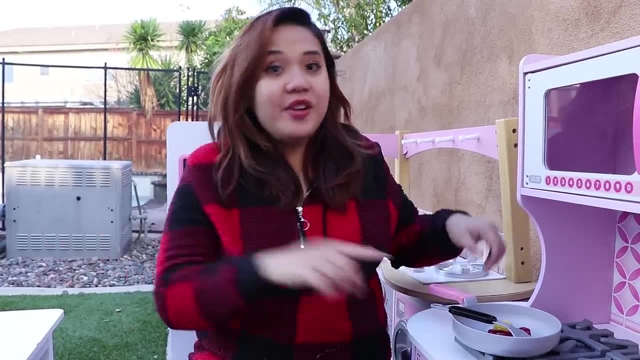 Come on, Liam, Hi Auntie Rose, Hi Wendy, Liam, What have you got here? Do you got any food? No, we're not hungry, We're looking for letters. Have you seen any Letters? Oh, I found some right here. Wow, so cool. 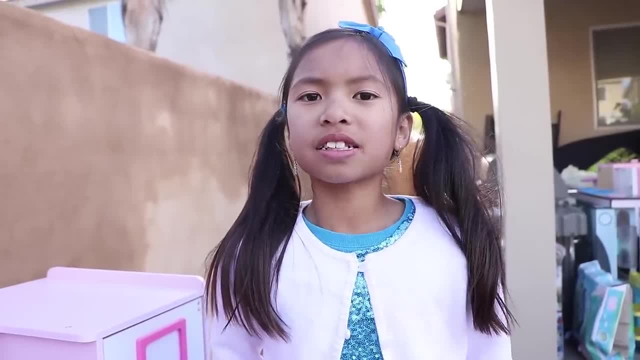 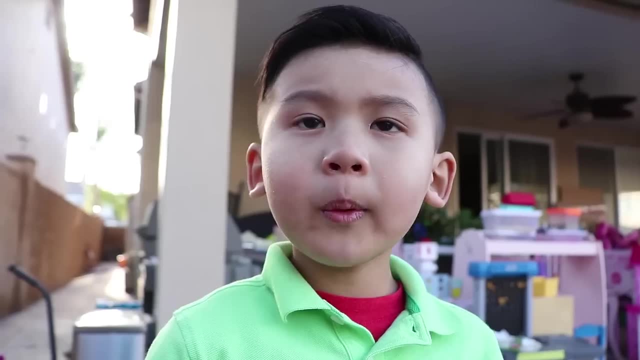 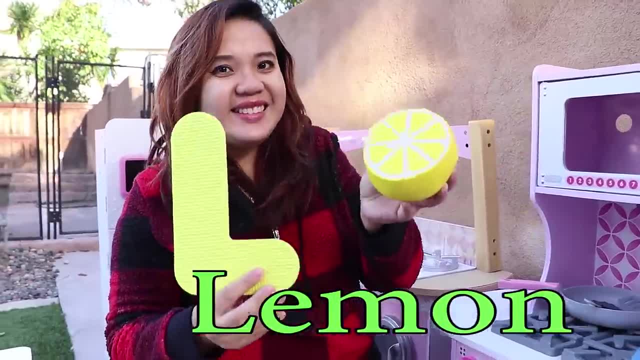 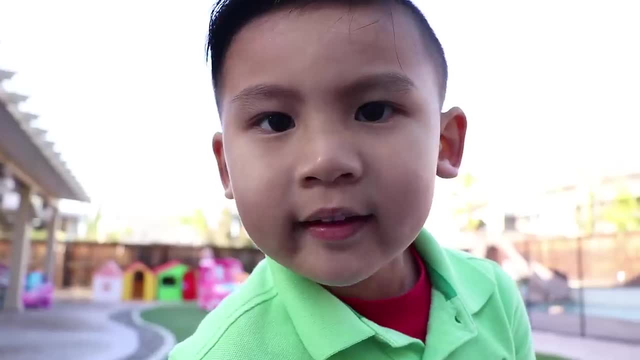 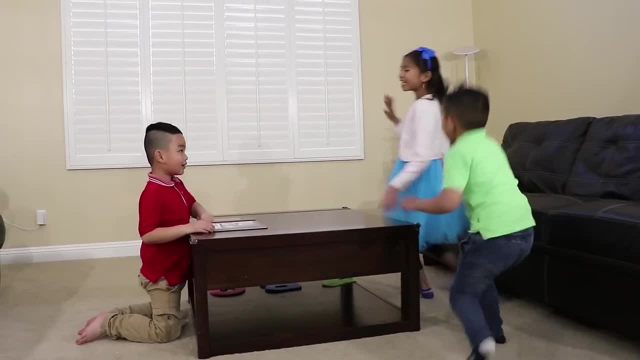 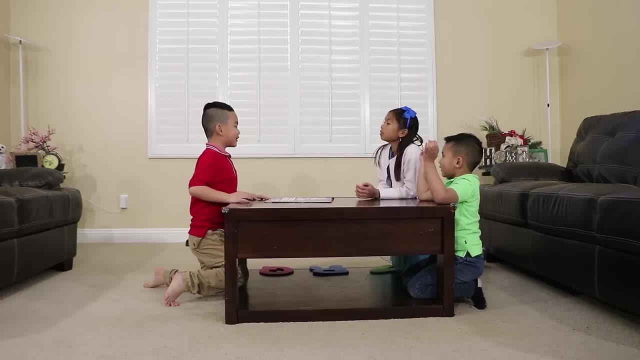 Liam, let's go find more letters. Okay, Bye Auntie, Bye Hi Lindy, Hi, Hi guys, What do you need for letters? Did you see any? No, my people, Let's go find it. Okay, Ah, I found some letters. 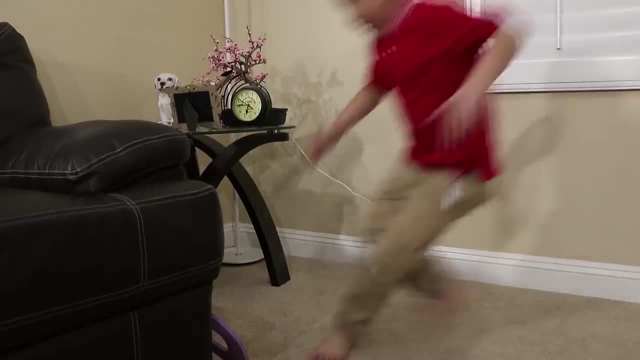 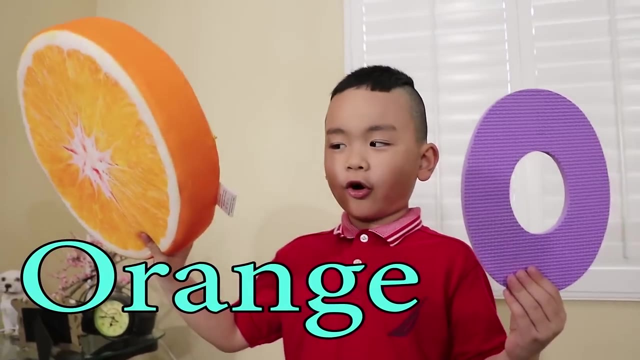 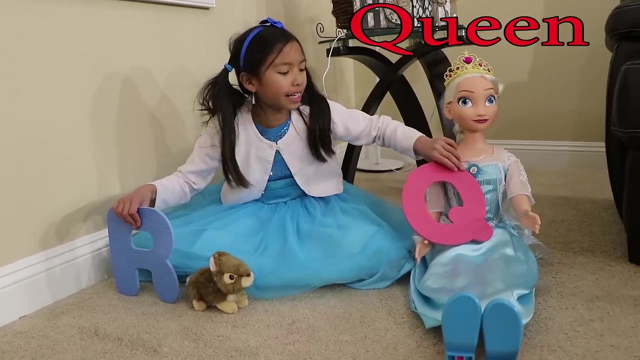 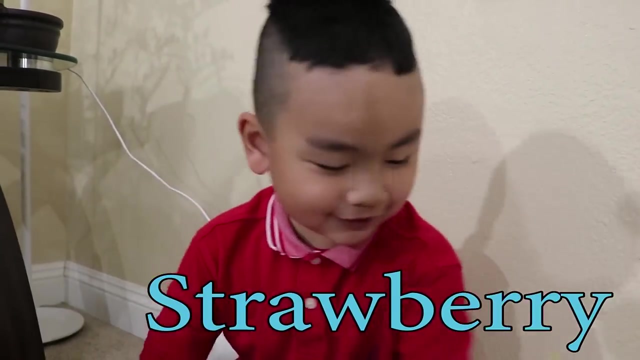 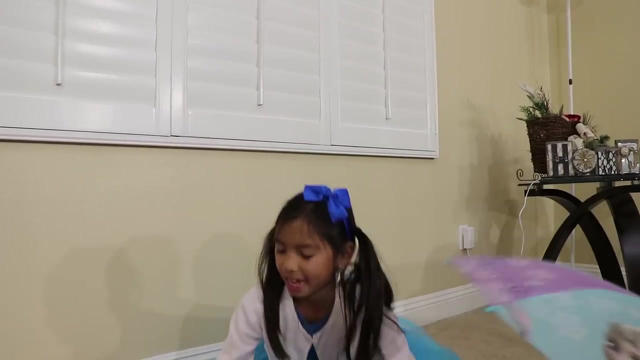 right here. I found some too. I found some letters: O is for orange and P is for pizza, Q is for queen and R is for rabbit, S is for strawberry and T is for toothbrush, U is for umbrella and V 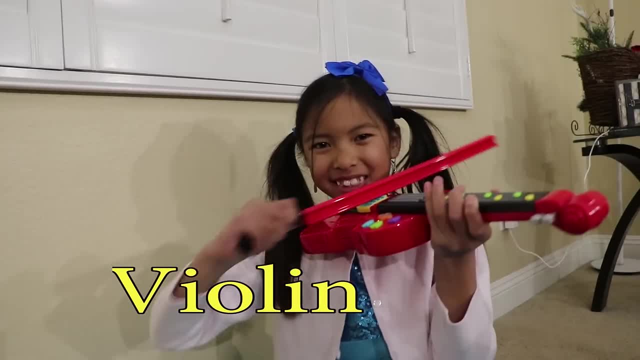 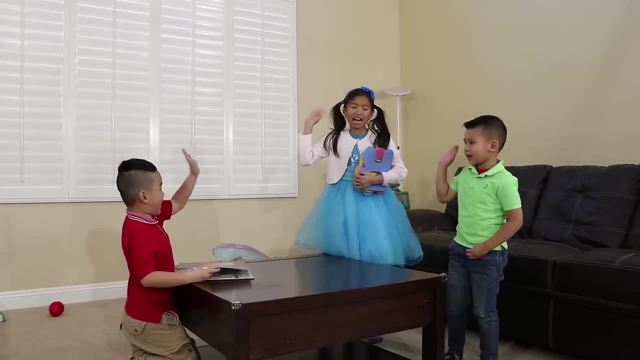 is for violin. Yay, Got it, Thank you. Let's go find more letters, Liam. Okay, Thank you, Landon. Bye, Hi Uncle Tim, Hi guys, What do you guys need? We're finding letters. 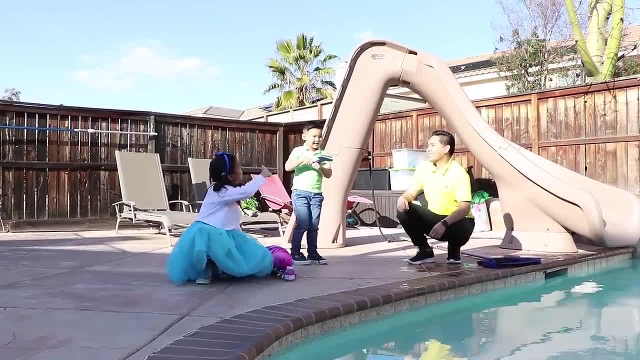 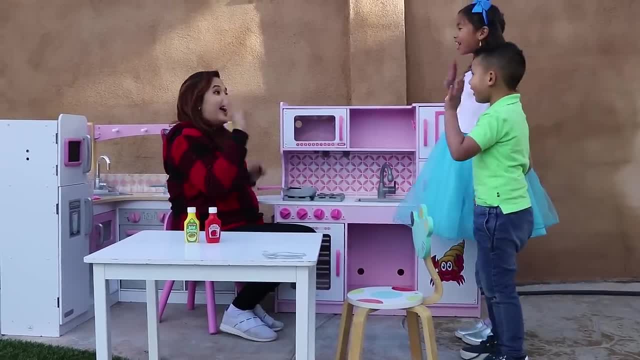 Let's go find more letters, Liam. Okay, Thank you, Uncle John. Bye, Bye guys. Come on, Liam, Hi, Auntie, Rose, Wendy, Liam, What are you guys here? Do you guys need food? No, we're not hungry. 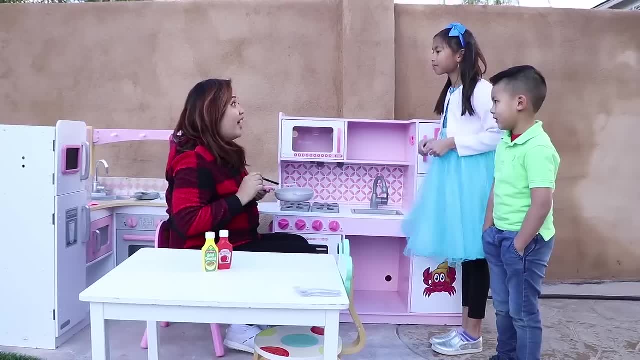 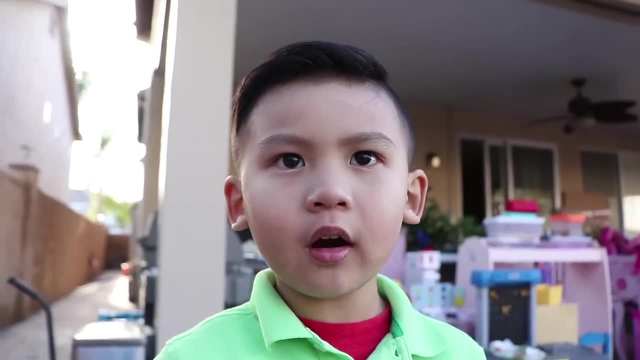 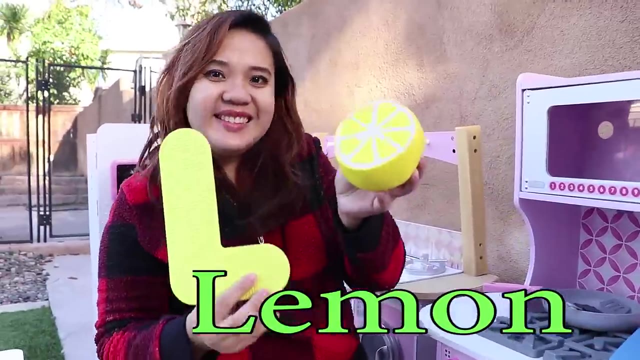 We're looking for letters. Have you seen any Letters? Oh, I found some right here. Wow, so cool. Where are these letters? Hey, Liam, Let me show you Letter K for kitchen and L for lemon. M is for motorcycle. 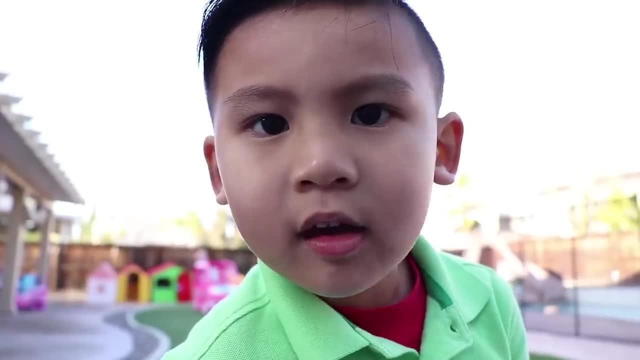 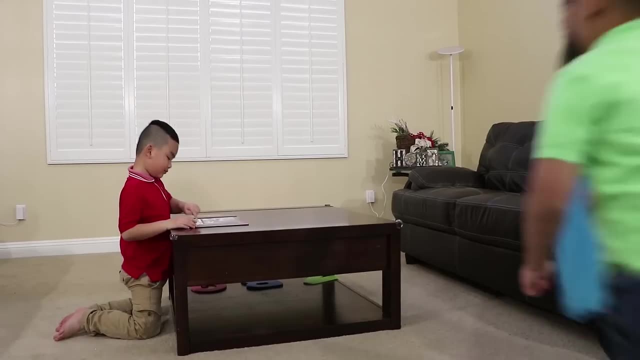 N is for necklace- Awesome, Thank you, Wendy. Liam, let's go find more letters. Okay, Bye, Auntie, Bye Hi Wendy, Hi, Hi guys. What do you need? We're looking for letters. 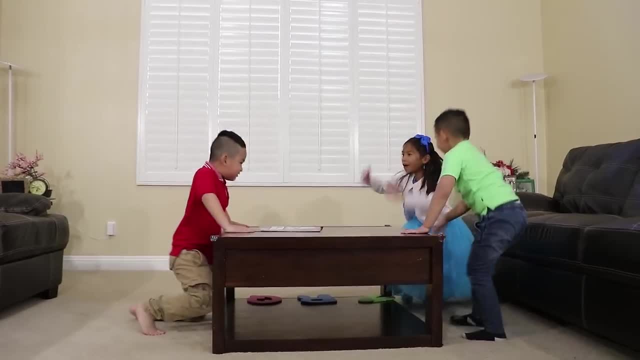 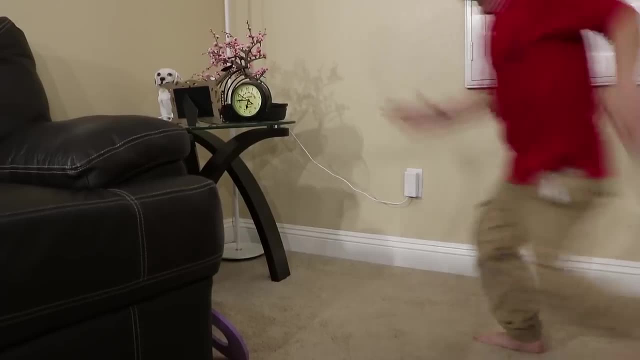 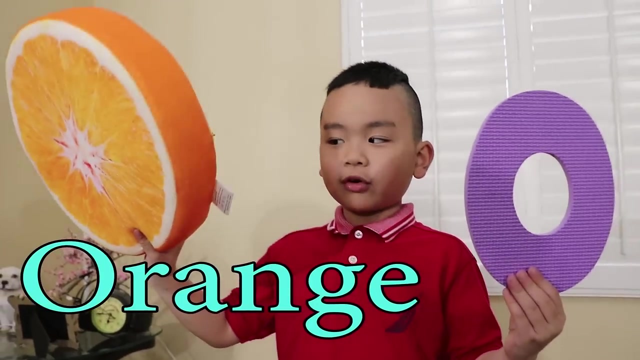 Did you see any? No, Wendy, But let's go find it. Okay, I found some letters right here. I found some too Cool. I found some letters: O is for orange and P is for pizza, Q is for pizza. 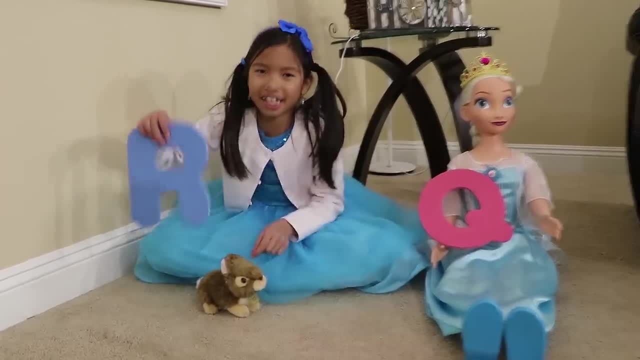 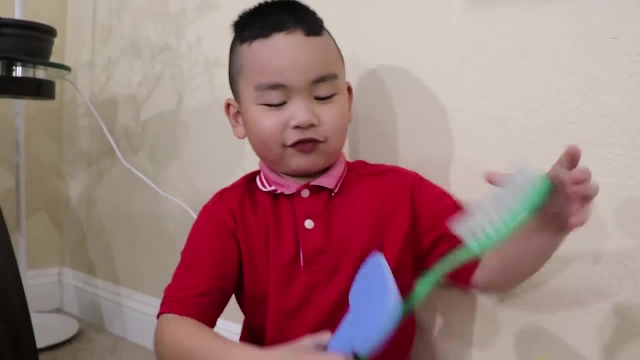 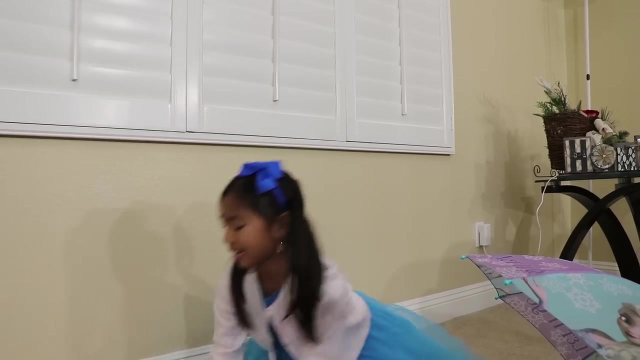 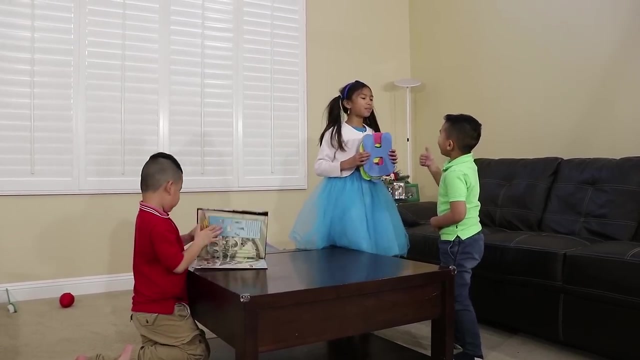 Q is for pizza, A is for queen and R is for rabbit, S is for strawberry and T is for toothbrush, U is for umbrella and V is for violin. Got it, Thank you? Let's go find more letters, Liam. 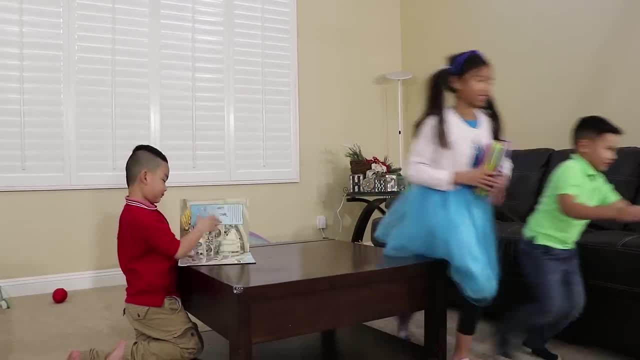 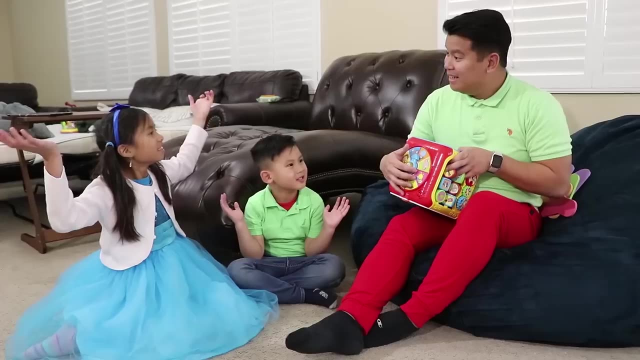 Okay, Thank you, Lyndon, Bye, Bye, Bye, Uncle Tim, Hi, Uncle Tim, Hi guys. What do you guys need? We're finding letters. Did you see any Letters? Yeah, I found some earlier. 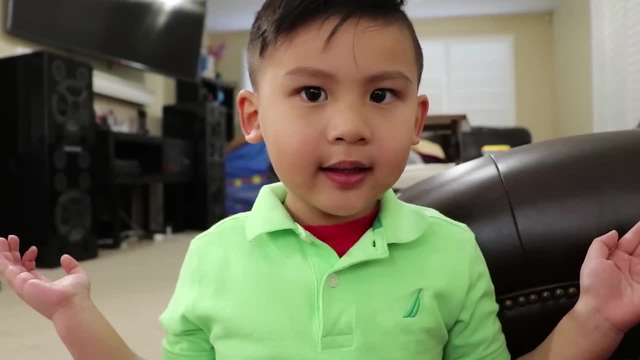 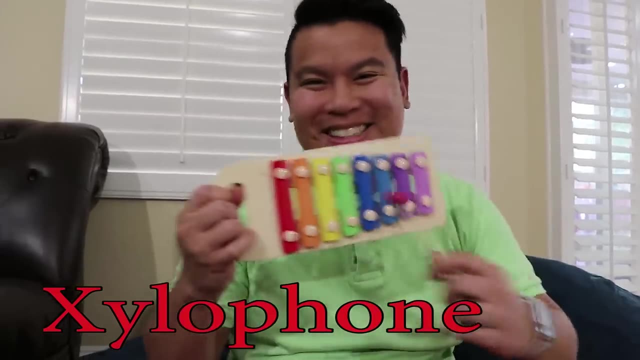 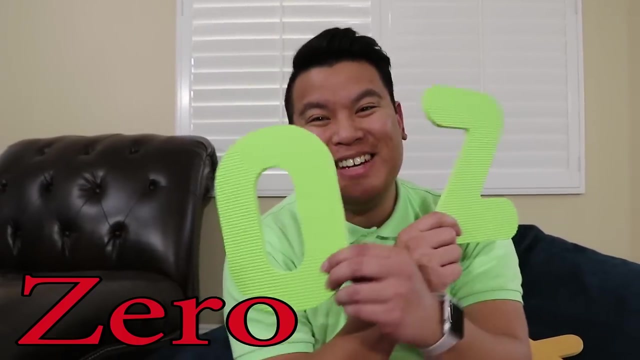 Is it these? Yeah, Where are these letters? The letter W is for wand and X is for xylophone- Check it out- And Y is for yogurt. And the last letter is Z for zero. And let's go take them back.